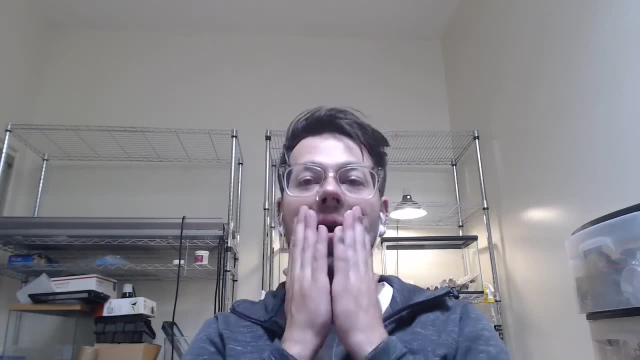 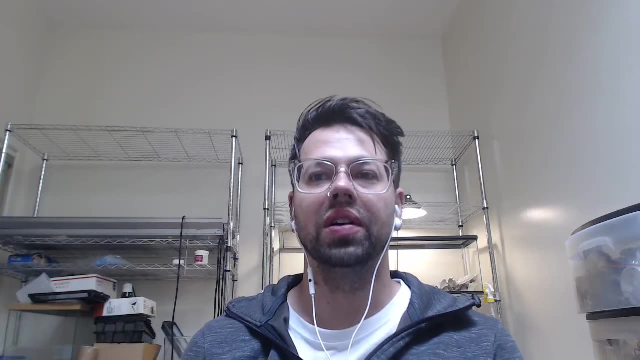 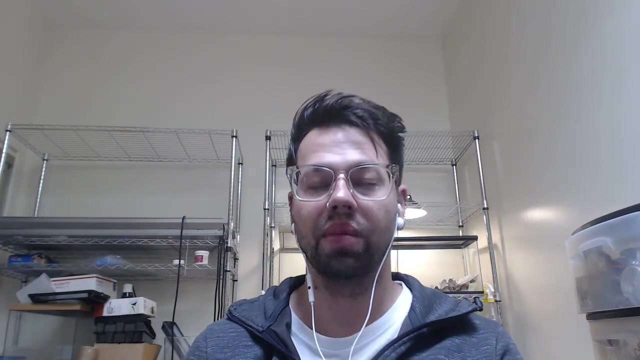 So, um, Scientists use them all the time. Now, one of the things that we're going to discuss today, and is pretty much the main way to do genetic engineering, is by using plasmids. Plasmids- We're going to talk about that today. 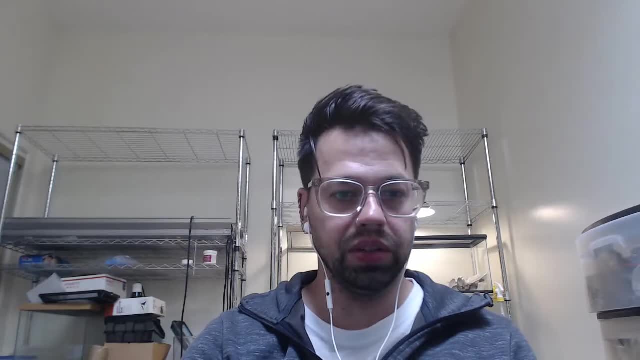 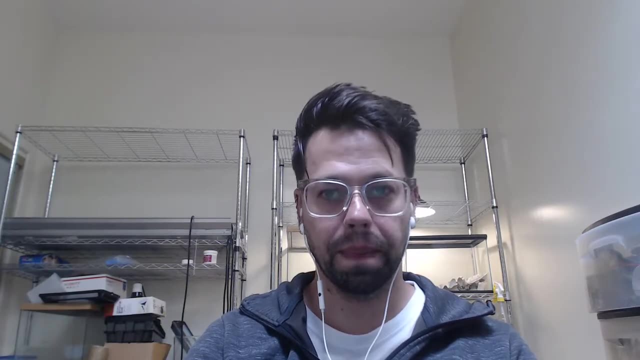 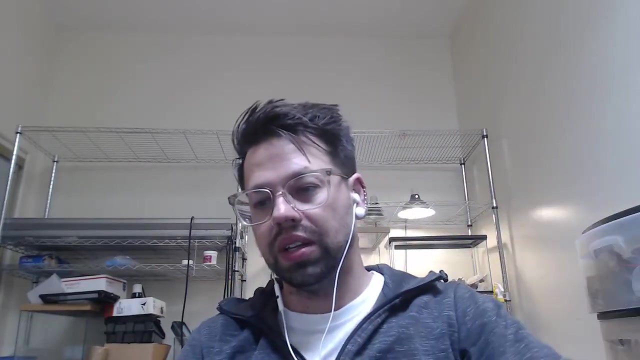 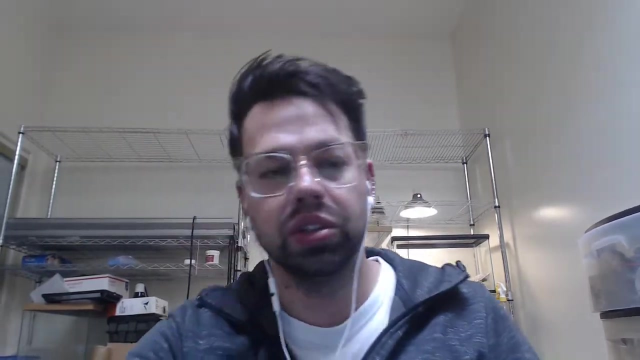 Okay, actually what I might do is first do a little bit of some drawing so that I could just, you know, kind of explain what's going on with the plasmids and DNA and genetic engineering. Then, if you haven't already make sure that you download Snapgene. 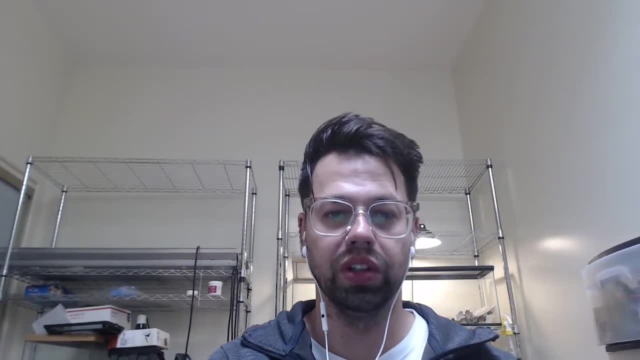 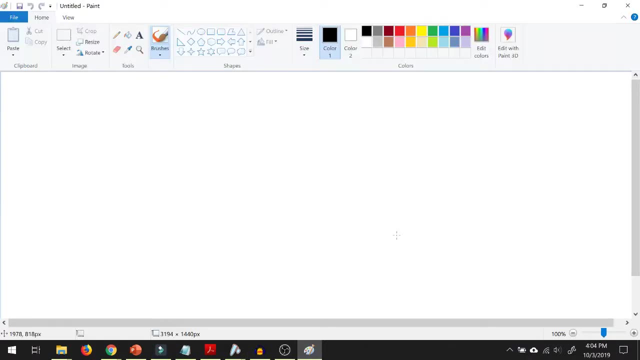 Snapgene is what we're going to use later today to look at what's actually inside of plasmids and how plasmids work and all that good stuff. So while you're- you know- following along today, go download Snapgene. 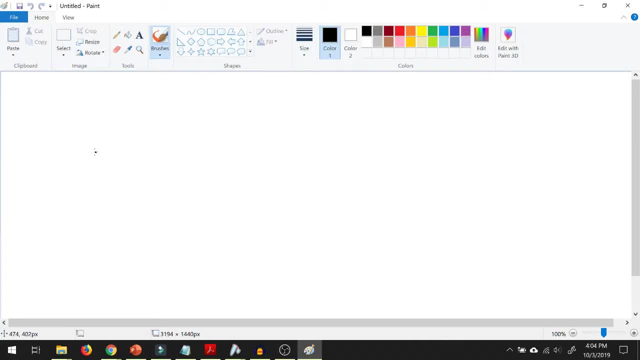 Snapgene Viewer. It should be free, All right. All right. So let's say we got a bacteria and it's got a flagella and it's just like swimming along and stuff like that. So the bacteria has its own genomic DNA in there, right? 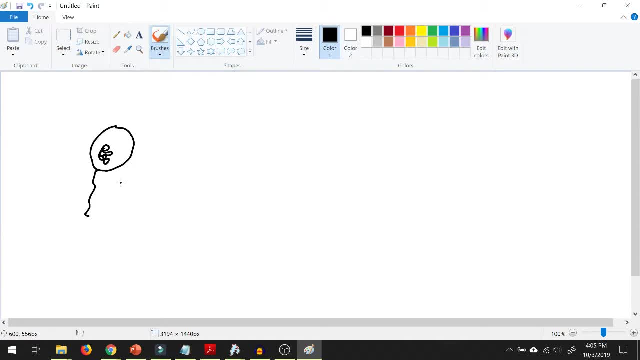 It's really big. the genomic DNA of bacteria. It's like three million base pairs. let's say, Now in science there's this thing called a plasmid. Now plasmids naturally occur. Plasmid is a piece of DNA that's generally around 2,000 base pairs to maybe like they can be pretty huge, but generally they're between 2,000 base pairs and like 20,000 base pairs, right. 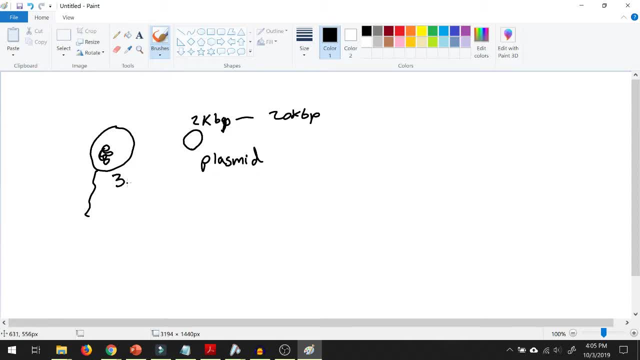 And the genome of the bacteria. So what happens is these bacteria will store these plasmids because they can transfer them easily between different bacterias. They can pick them up. It's just something that evolution has created that allow bacteria to transfer genes, you know, between species. 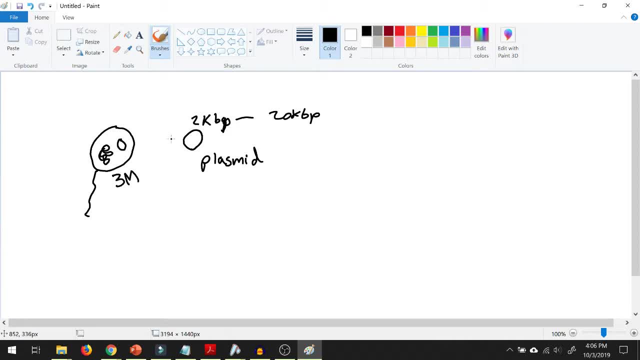 And between other bacteria really easy. So generally, when you're working with plasmid DNA, the goal is to get the plasmid DNA inside the organism, whether it's bacteria or yeast, or human cells or fungi or animals, whatever right. 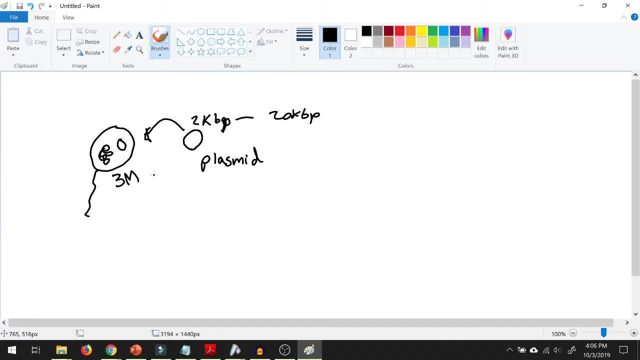 You're trying to get the piece of DNA inside bacteria, So That's all you're worrying about. That's your only goal. Once the piece of DNA is inside bacteria, it has genes on it that tell the bacteria to replicate the plasmid and do certain instructions that you want it to do. 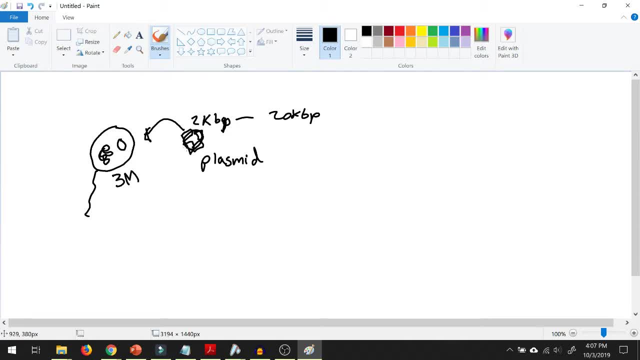 And people code that themselves. So they code the DNA and you could code the DNA yourself to get the bacteria you want to do Now. Generally, the ways to get the plasmid inside bacteria involve adding certain chemicals. The chemicals that are usually involved are polyethylene glycol in bacteria and yeast. 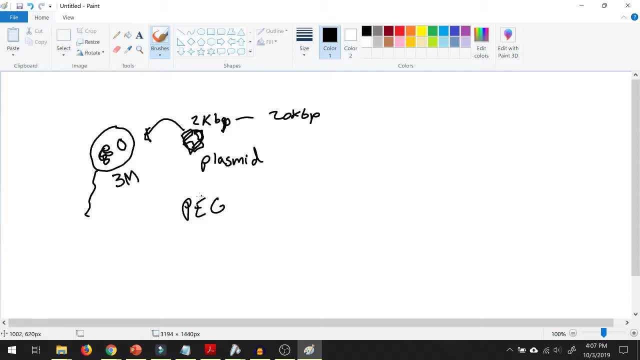 And what PEG does polyethylene glycol is it helps open up the bacterial membrane And what PEG does polyethylene glycol: is it helps open up the bacterial membrane? Right, Because polyethylene glycol is a polymer that will interact with the non, with the lipid membrane of the bacteria. 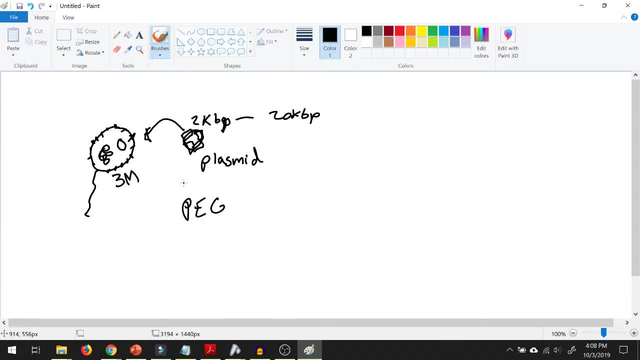 It kind of creates pores and holes in it And this helps the DNA get inside the cell Right Usually. there's also another chemical which Is a positively charged cation And bacteria use calcium chloride And yeast use lithium chloride. 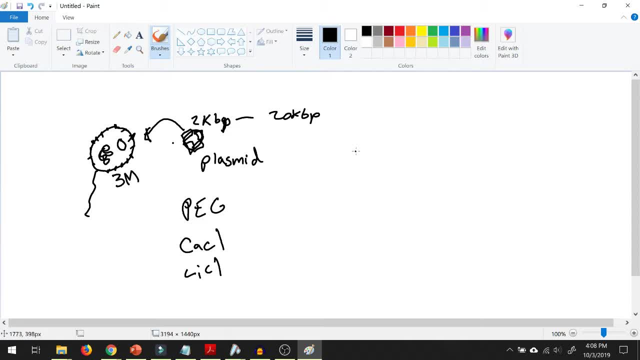 And what this does is plasmid DNA. any DNA is usually negatively charged Right, And so the positively charged cations right- Calcium lithium. What they do is they help neutralize the charge of DNA, So it becomes more inert. 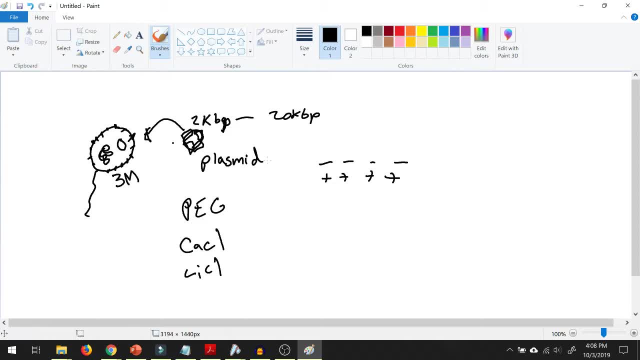 And that makes it easier for it to travel Through membranes and things like that Right. So generally those are the two big parts of the transformation. PEG and calcium chloride, All you generally do in most transformations, whether it's human cells or bacterial cells or yeast cells. 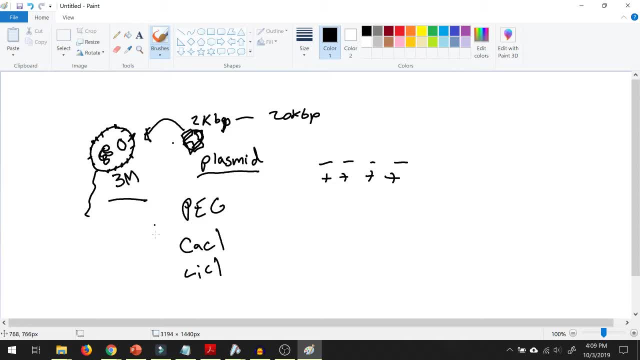 is mix the plasmid, the organism and some chemicals, And that's literally it, And then you just let them do their thing, And that's what is involved in a transformation. All right, So the transformations that you are going to do are very similar. 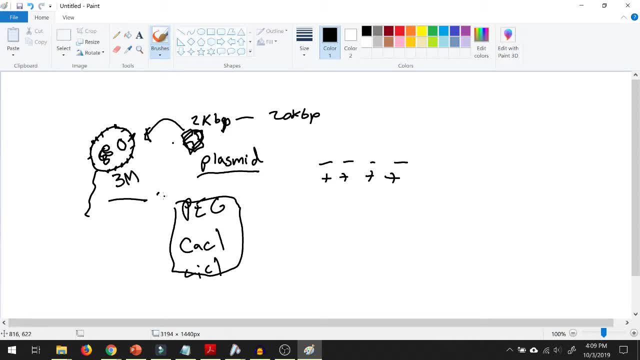 What you're going to do is you're going to mix some bacteria. The fresher the bacteria, the better. The fresher the organism. right, The organism's healthy. It's going to be robust. It's going to keep growing. 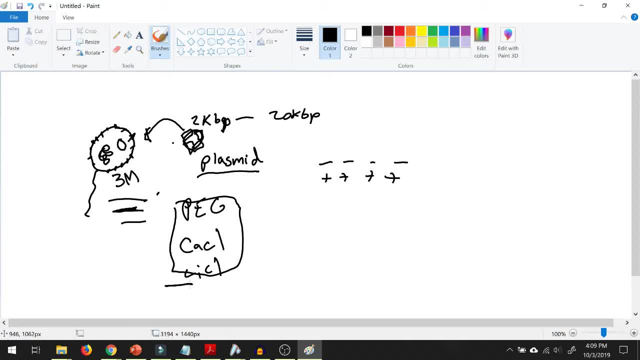 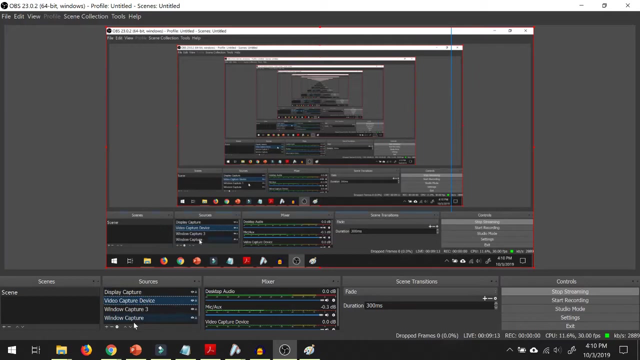 So fresh bacteria And mix it with the bacterial transformation mix And mix it with some plasmid DNA And hopefully at the end you get a GMO Right. So what is First off? do we have any questions? 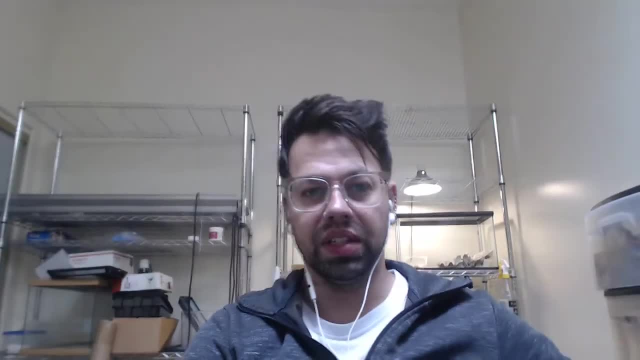 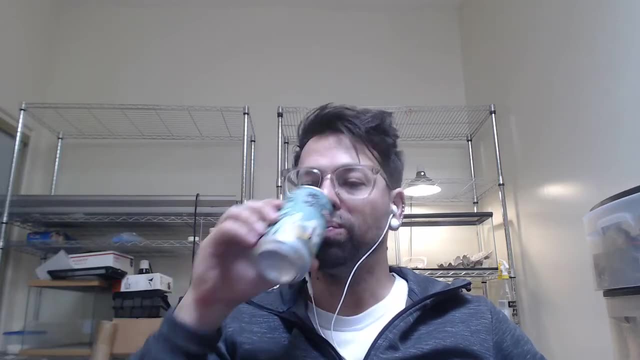 Any questions on any of that stuff That make sense. You just got some DNA And you're just trying to shove it inside an organism. Shove that DNA inside the organism And get the organism to use it, Basically when you're doing transformations. 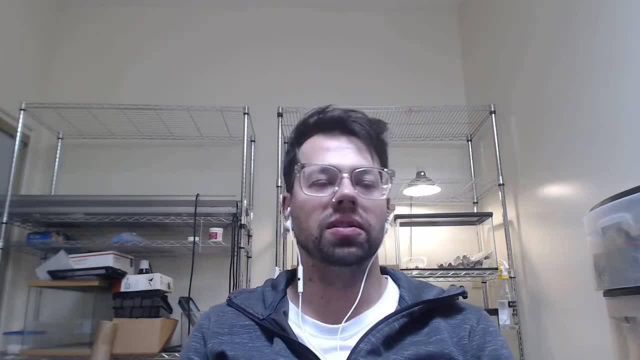 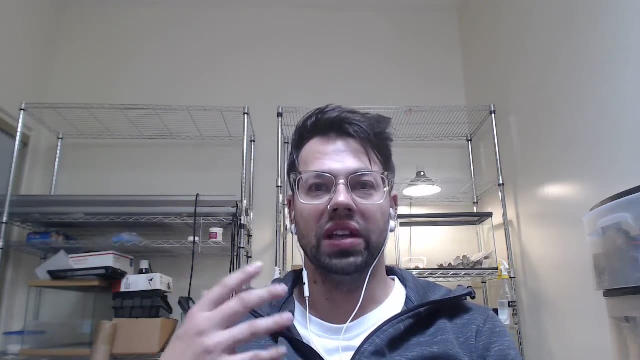 what you're trying to do is, you know, kind of like hack the organism. You're trying to convince the organism that the DNA you're giving it is its own DNA. So then it'll replicate it, It'll make the proteins. 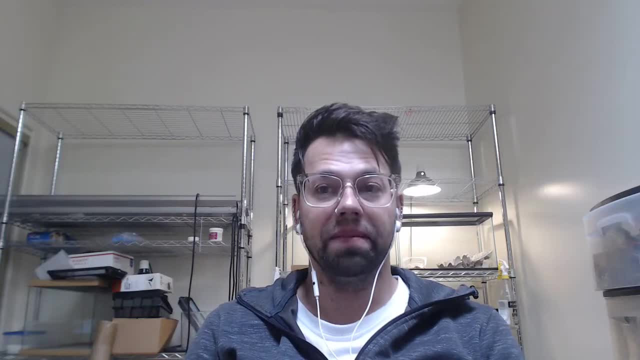 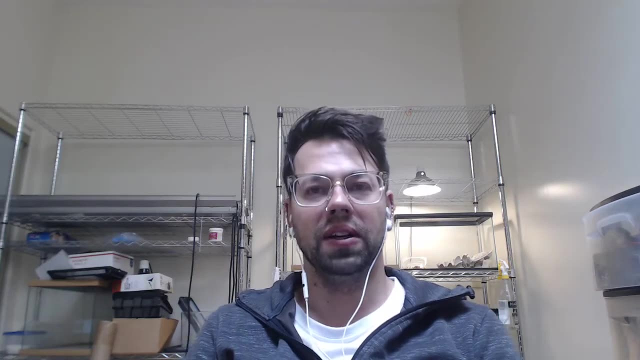 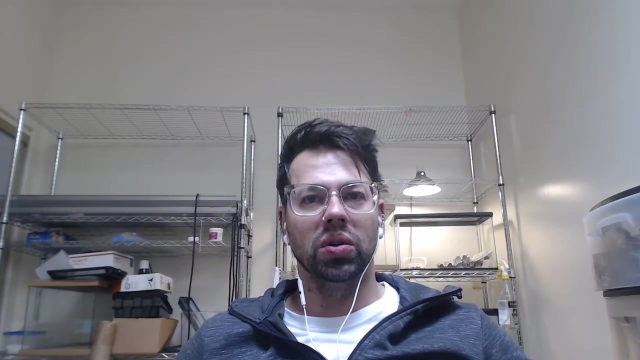 And It will think It's its own DNA. That's basically the goal, And we figured out kind of like standardized things that you need to include for this to happen. But that's basically the goal of the transformation. Is tricking the organism? 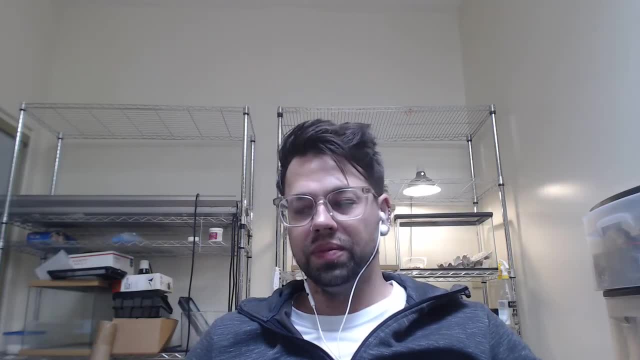 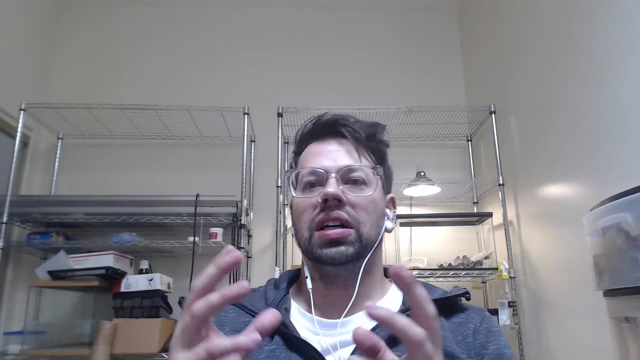 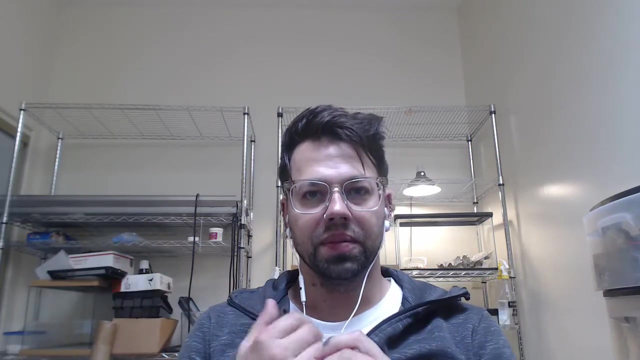 Into thinking that it's its own DNA. So when you're trying to use DNA Between like bacteria and yeast and humans Generally, it won't work Right. So bacteria have different control elements in their DNA Than yeast. 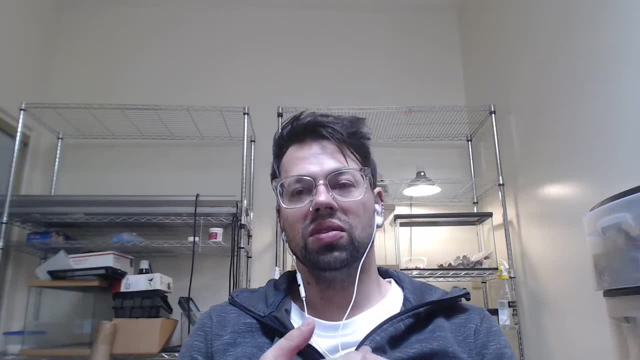 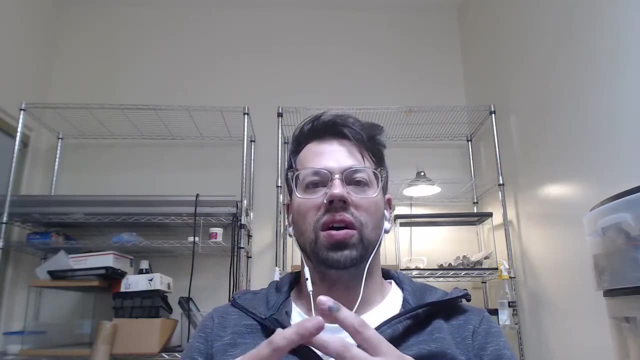 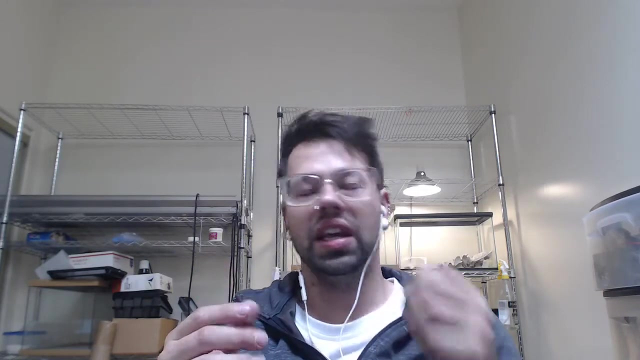 Than plants, Than animals, Right? So all these organisms have different control elements in their DNA That allow the DNA to work properly, To tell it exactly what to do. So a piece of DNA, As we, you know, learned about. 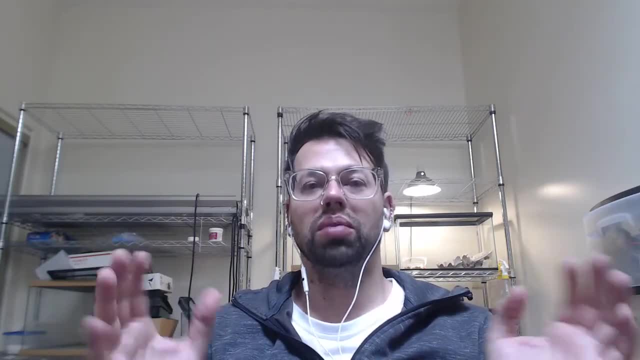 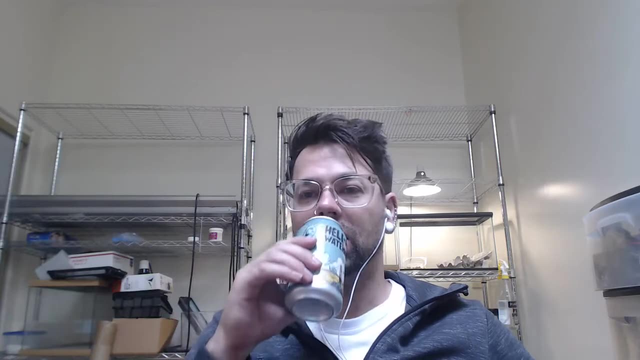 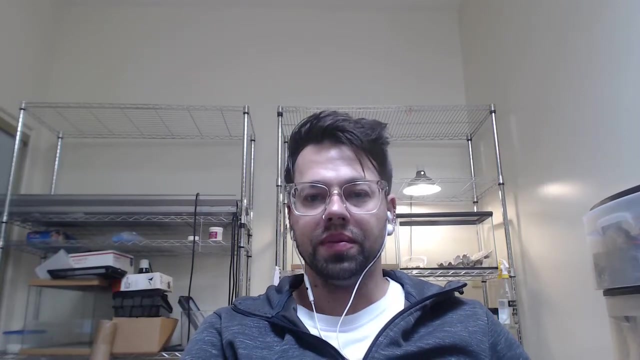 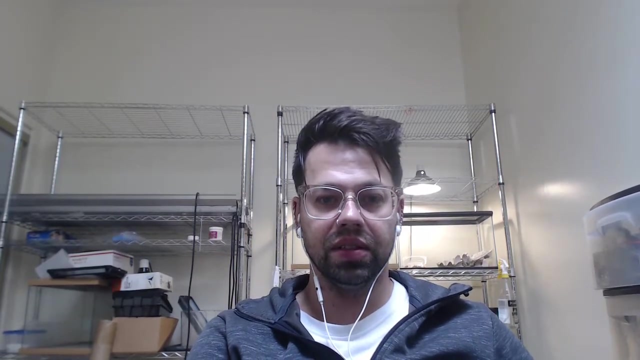 Isn't just like telling you that it should make a protein. There's so much more that actually goes into it, And we'll talk about that in a second. Yeah, Alright, So Let's Look at SnapG. 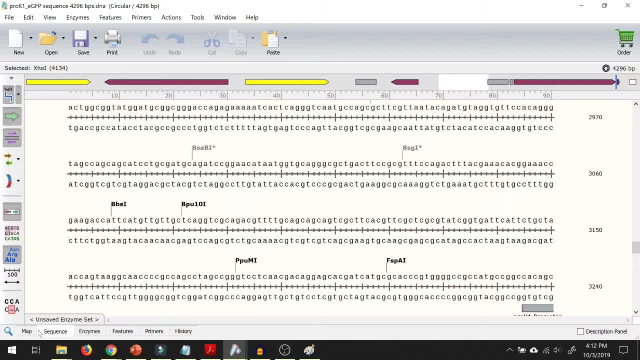 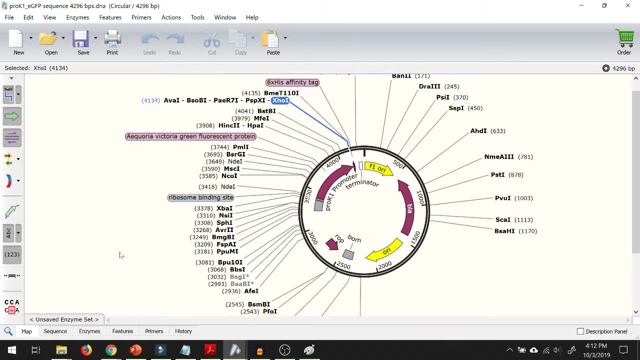 Download SnapG. I think on the Google Classroom there should be some DNA sequences. Download the DNA sequences, Open them up And Let's look at what a plasmid Piece of plasmid DNA looks like, If I have this set up properly. 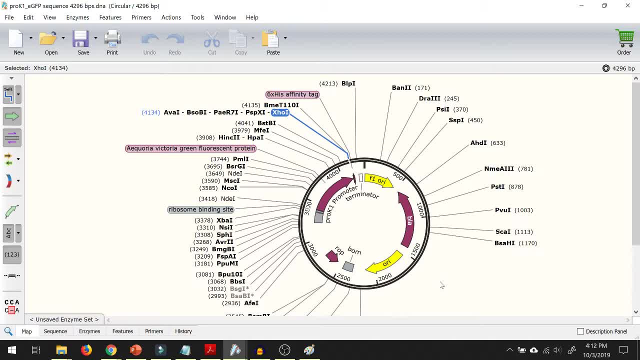 So this is a piece of plasmid DNA, Okay, And This is what we call a plasmid map, Right? So a plasmid map contains All the major DNA elements that are on the plasmid. 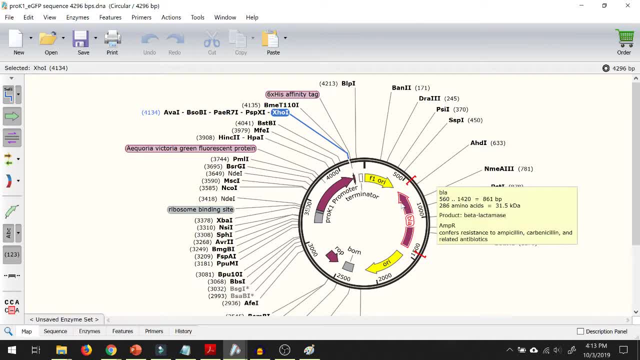 And which direction they are being transcribed, So Which strand is being used? So If it's going this way, it's the top strand, Right? If it's going this way, it's the bottom strand. So It's easy to figure out what these things are. 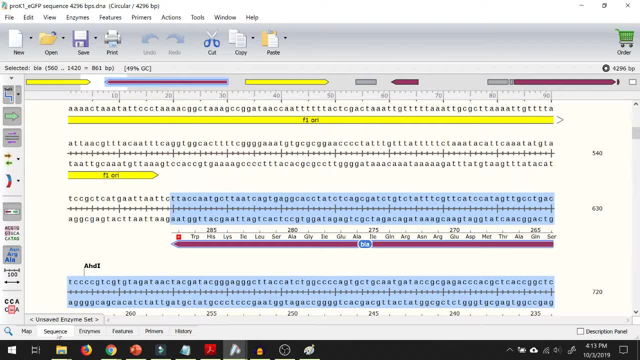 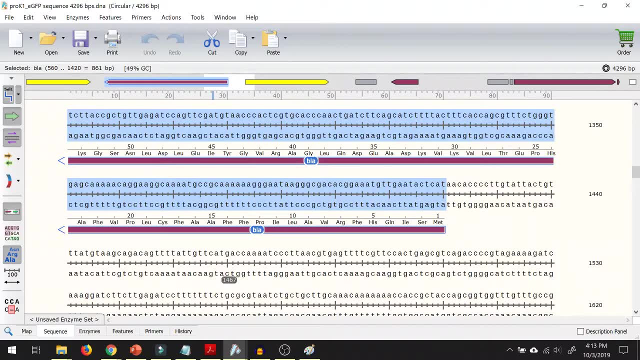 We can just look at the sequence Right And see what's actually coding for it. So we can tell here the methionine amino acid is coded for by the codon ATG. It's on the bottom strand, going in the 3' to 5' direction. 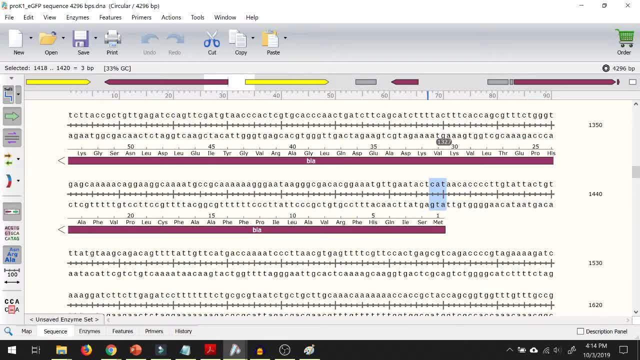 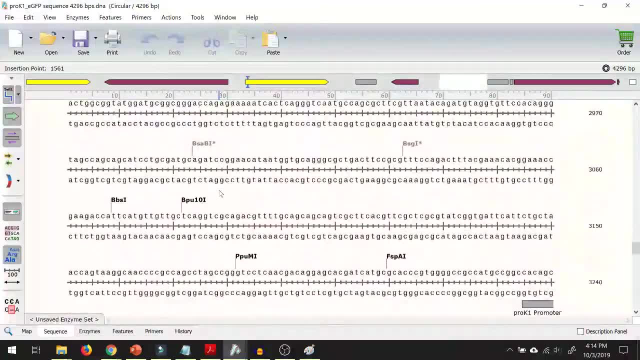 Right, So that's that gene. And now if we go over to this one, Actually that's an origin of replication, It's not a gene. If we go over to this gene, you can see the same thing. ATG. 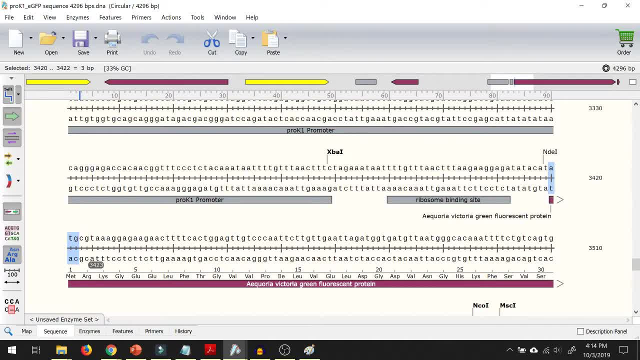 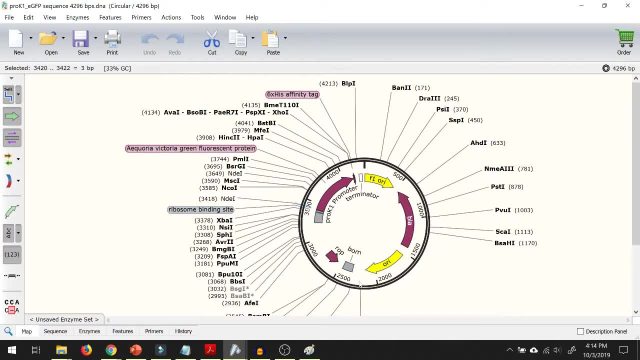 ATG, Except it's going. It's on the top strand And it's going in the opposite direction, Right So? But you don't have to worry about that stuff too much. That's probably more technical stuff That You won't really have to need to know if you're just getting started in genetic engineering. 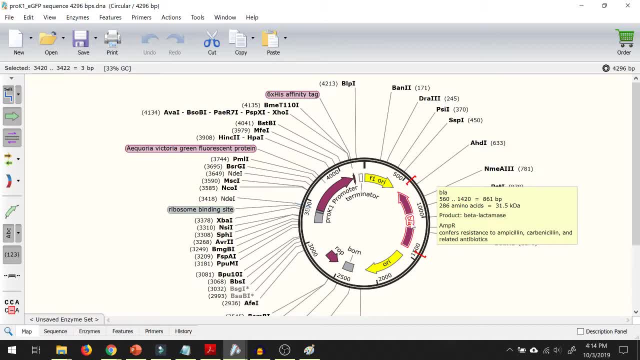 Or doing genetic engineering with plasmids or things like that. Generally, you just want. You just want to know where your gene is, And that's it. All this other stuff in the plasmid is not that important. Well, it is. 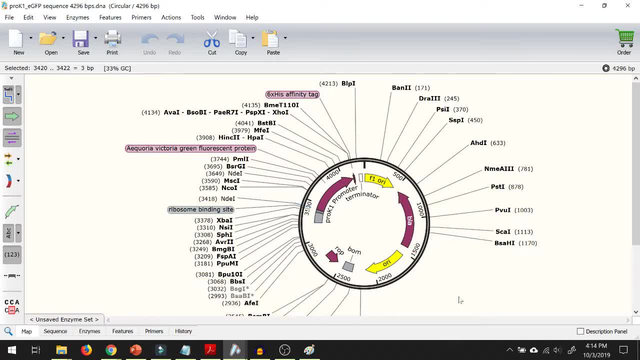 But it's not So. a plasmid is composed of a few main things, Generally what we call everything. that's not the gene that you put in. So in this case we'll say: the gene we put in is the green fluorescent person. 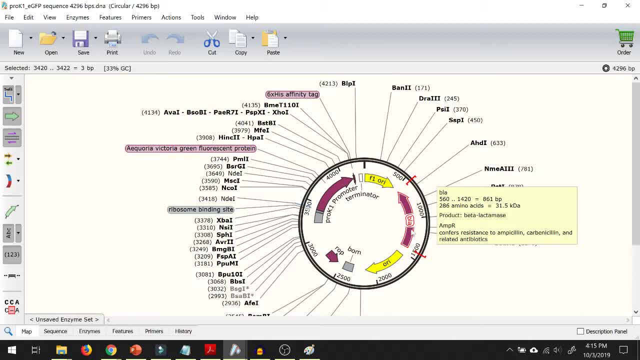 We call it the plasmid backbone Right, And the plasmid backbone is just all the junk that you kind of need for the plasmid to work Right. It's just all that extra junk that's sitting around that makes the plasmid work. 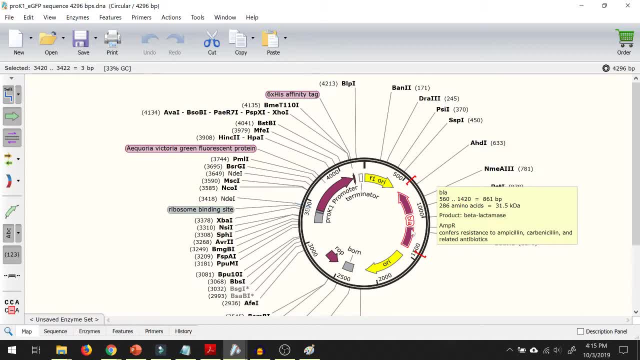 And so, Generally, you're not going to care too much. The one thing that you will care about is the antibiotic resistance gene. But the antibiotic resistance gene tells you how you select for your genetically engineered bacteria. So let's talk about this a bit. 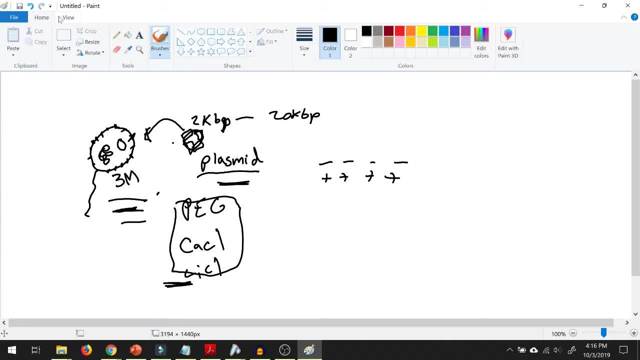 All right, Let's go back to this diagram Or drawing program. It's paint, I know. I know it's paint, Don't hate, Don't hate, I like paint, All right. So how does a genetic engineering experiment work? 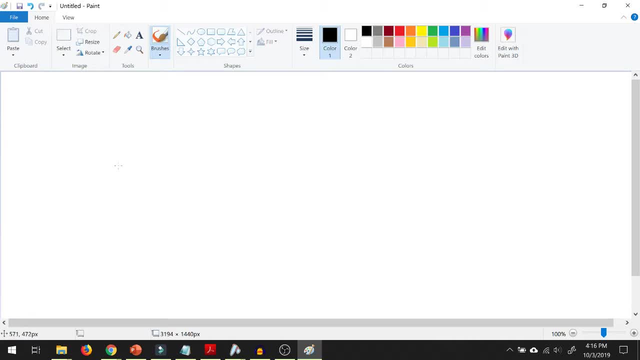 Now, this is the case for most all organisms, Right? So generally you have like a whole tube filled with bacteria, Right, Right, These are all little bacterias Inside our tube. We got our little micro centrifuge tube. 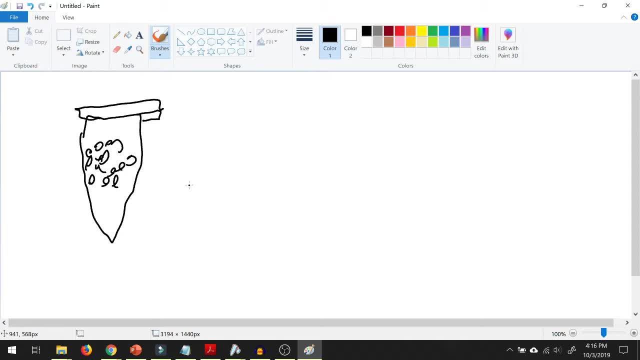 That's filled with bacterias. Right Now we add our plasmid DNA Right And that goes in there. So the plasmid is obviously not going to make it into every single bacteria. There's a certain efficiency of the transformation. 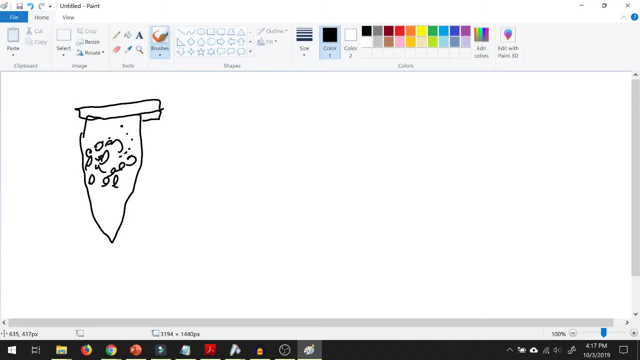 So only some of the bacteria are going to be engineered. Well, how do we know which bacteria or yeast or human cells get engineered? The thing is, is you include an antibiotic resistance gene, And usually people write this as like ampicillin. 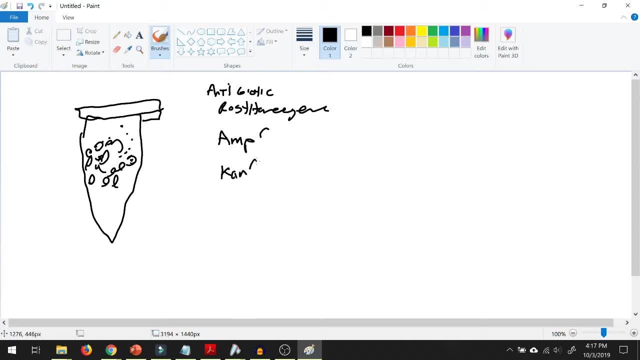 Ampicillin resistant, Canomycin resistant Or something like that. So what you do is, after you add the DNA and mix it with the bacteria, you put it in media, Generally a petri plate that has some antibiotic in it. 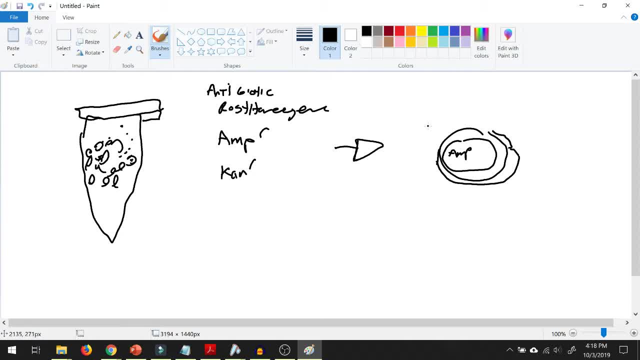 Right, Ampicillin. Now what happens is, if you put the bacteria on here, the ones that didn't get the DNA are going to die Because they don't have an ampicillin resistance gene from the plasmid. The ones that got the DNA are going to live because they also have the ampicillin resistance gene from the plasmid. 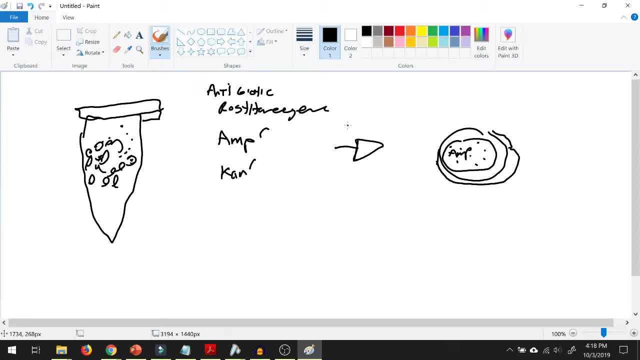 So it's a really simple assay where you can determine, you know, what is genetically engineered and what is not genetic. Now, the same technique is used for everything: It's used for plants, It's used for human cells, It's used for yeast. 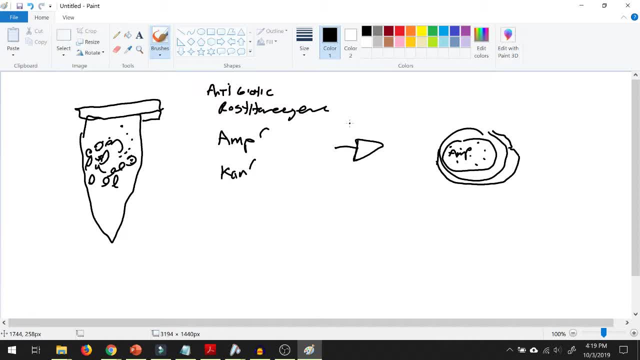 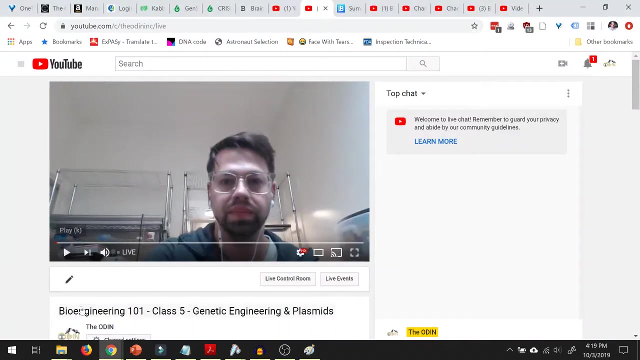 It's used for everything. You use antibiotic resistance genes. It's just the way that is easiest to kill off all the cells that aren't genetically engineered. it's as simple as that, right. so antibiotic resistance genes are in almost every single plasmid that exists. all right, we have any questions? no, no. 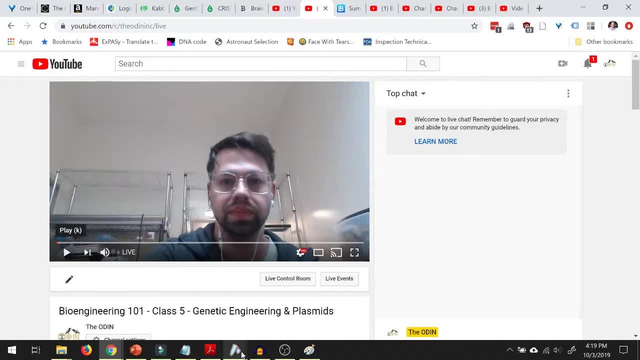 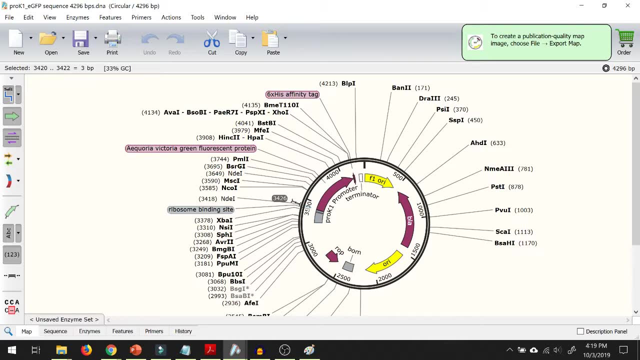 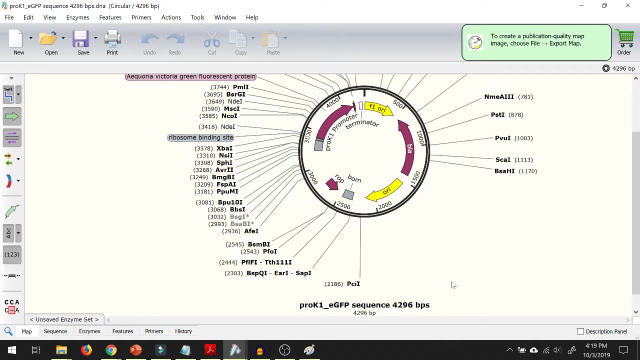 questions so far. okay, let's go back to the snap gene. all right, so we got our DNA sequence right here. we got our plasmid map. so really, the major thing that you are going to be interested in, the backbone that you're going to care about, is the antibiotic resistance gene. what is the antibiotic resistance gene? 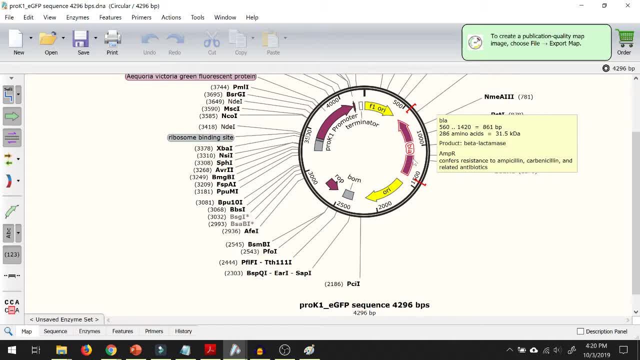 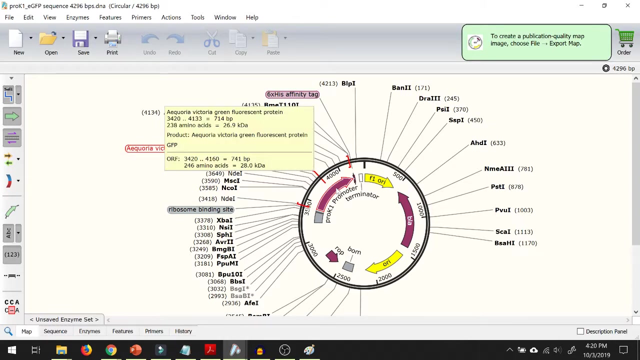 so you can use that specific type of media to select for bacteria that have been, or an organism that have been, engineered for this plasmid. so, besides that, all you care about is putting your gene in this plasmid. right here is an antibiotic resistance gene. however, you want to go ahead and do a. 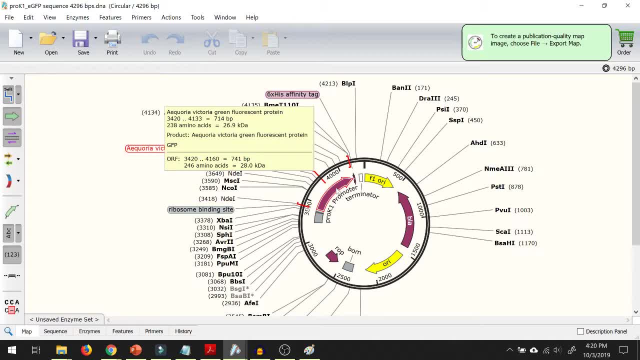 close test. you can use this gene or you can use any other gene here. you can even use this for being a local gene. here you can use all these different food sources. you can use this for food, all those different types of foods. you can use these for all of your ways of doing things like taking a blood test or 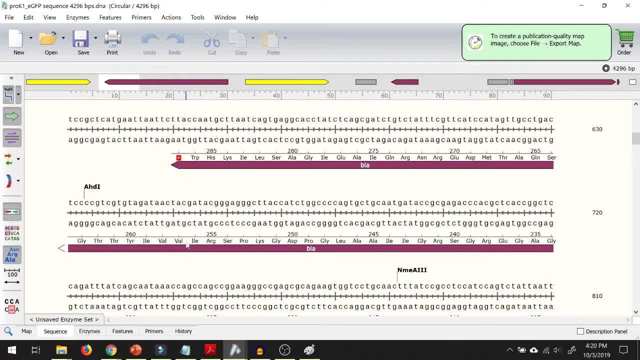 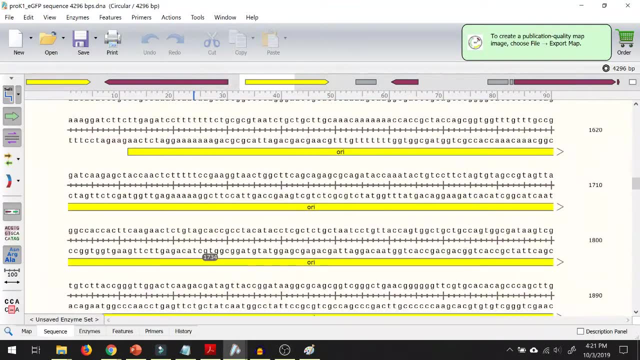 just taking an NOW or a blood test and then you just click all of those things that you can use and that's it. so take a look, okay. so the next part in this page is the antibiotic resistance. and then we got our antibiotic resistance, benicillin. This ORI is the origin of replication. What it does is it tells. 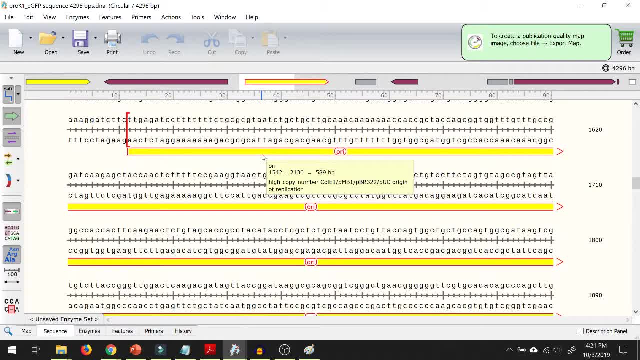 bacteria to replicate this plasmid. Yeast plasmids can also have yeast origins of replication. Generally, every plasmid- it doesn't matter the organism- is going to have a bacterial origin of replication because you replicate the plasmid in. bacteria, You can grow up large amounts of bacteria. and when you grow up these large amounts of bacteria, you can purify the plasmid DNA from them to use in other organisms. Otherwise, you can imagine trying, to, like, say, synthesize a piece of plasmid DNA is going to be expensive. 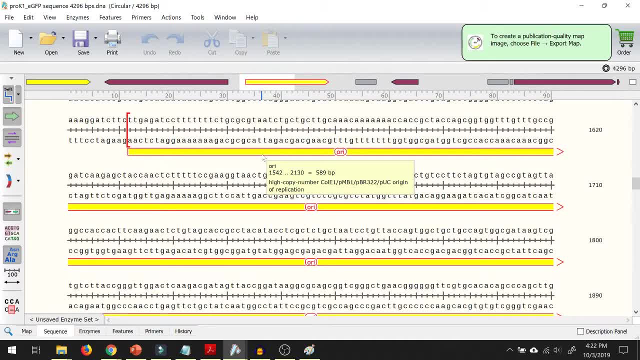 You know, Yeah, So we have learned to just replicate plasmids in bacteria. You can replicate them in yeast or something like that, but generally you're not going to get as much. Bacteria have the ability to create very high copy number inside their 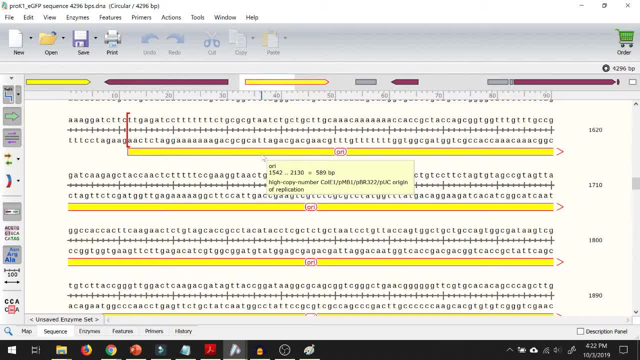 cells. So that means each bacteria doesn't have just one plasmid. Each bacteria might have hundreds of plasmids inside. Ok, So there are so many different copies of the plasmid inside the cell. Now, the origin of replication, depending on what origin of replication used there's. 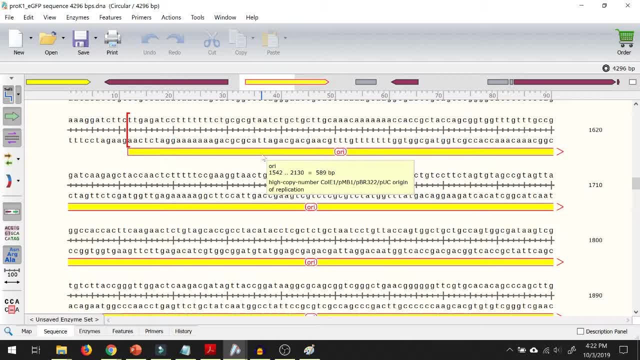 different origin of replications, The bacteria will create a different copy number of the plasmid in the cell. So there are what are called high copy number plasmids and low copy number plasmids and medium copy number plasmids. Now, what these copy numbers? 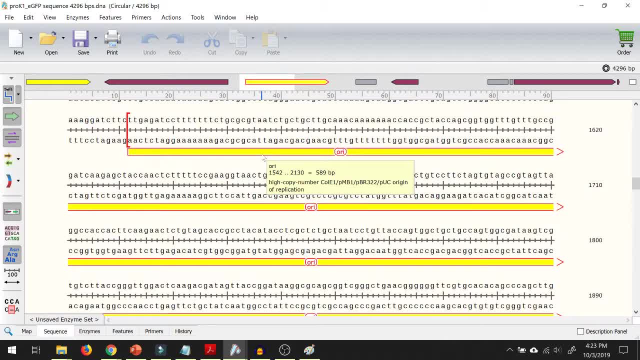 are. generally, it really depends what you're trying to do, right. If you're just trying to make, say, like a single protein and as much of it as you possibly can and the protein is not harmful to the bacteria at all. generally you want a high copy number, plasmid- As high copy numbers you can. 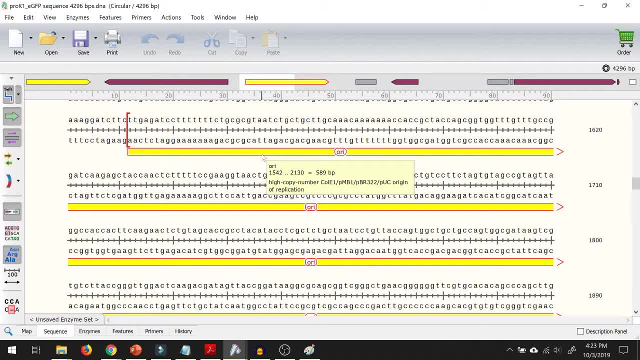 get, so that each bacterial cell will make as much of the protein as possible, because there's so many copies of that DNA laying around. Now it's not always the case that you want a high copy number plasmid. Sometimes you want a lower copy number plasmid, because 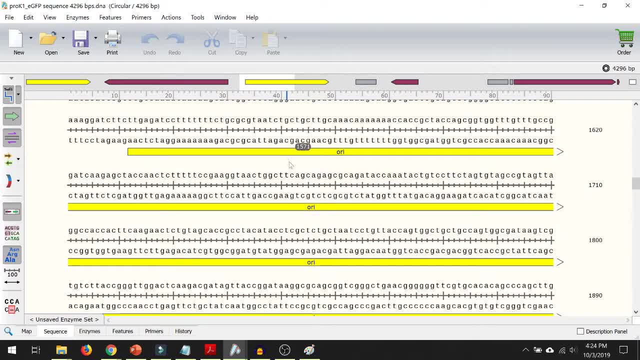 what you're trying to do is you're trying to express some protein that may be toxic. You're trying to express multiple proteins that are part of some metabolic pathway and, like. what you mainly want is you want the protein that is the rate limiting step to be expressed. 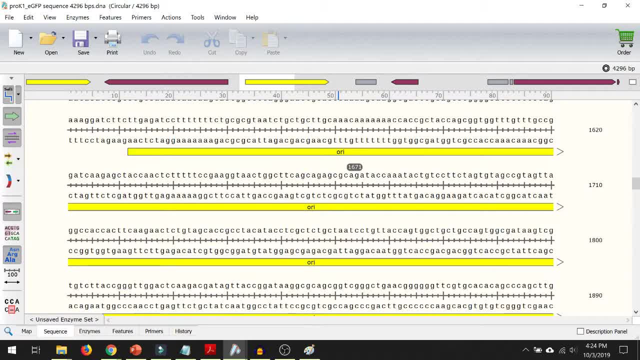 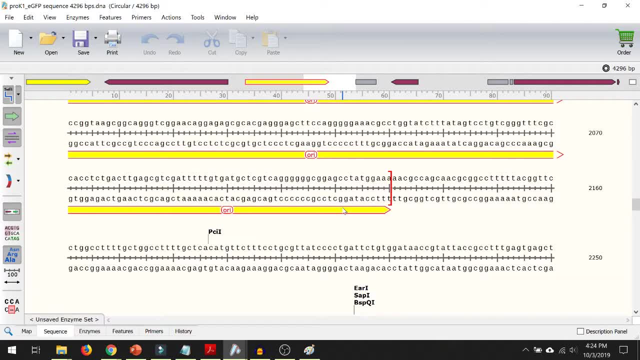 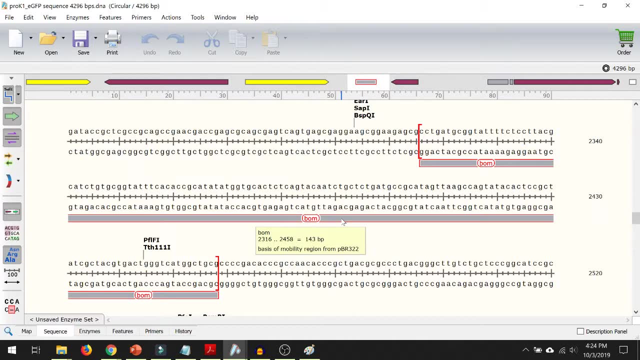 really high and the other proteins to be expressed lower because they don't matter so much. So there are cases where you may want different copy number of plasmids, but generally you're probably not going to deal with it too much. I don't think in my whole career so far I've ever tried to use a. 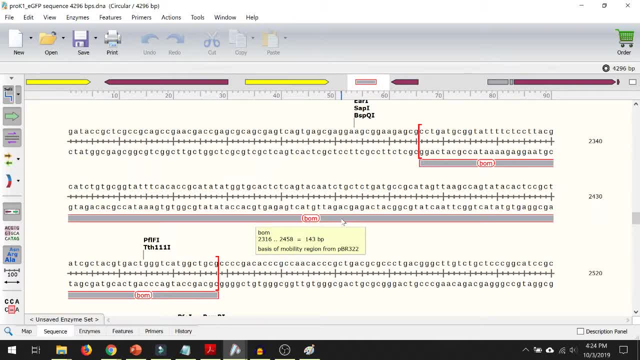 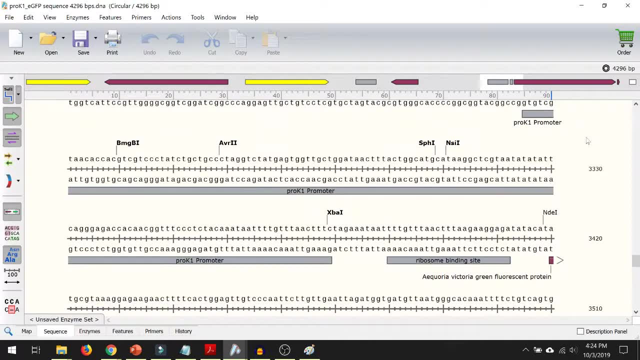 low copy number, plasmid or something like that, like on purpose. So you know, you may or may not, but let's just say probably not, we'll not have to worry about that. So what's after that? Now, generally, plasmids will have what's called a promoter. 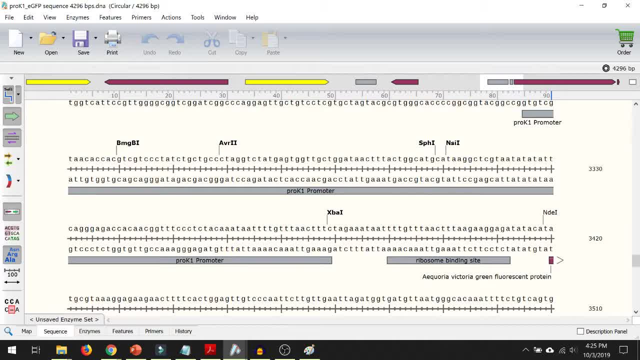 A promoter is a region that tells The RNA polymerase that it should bind and should start making the mRNA for this gene Right. So a promoter promotes the production Of mRNA for, for the cell. There are different types of promoters: promoters that create more and less. 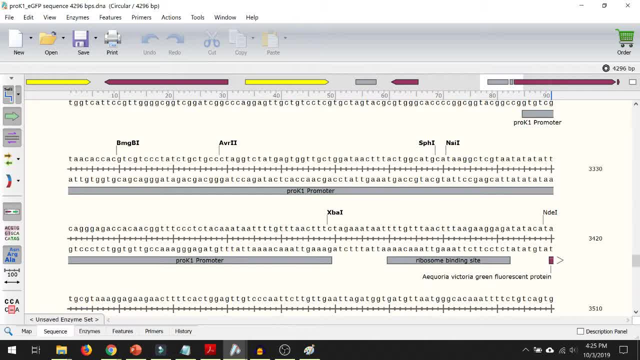 There are also things called enhancers and other things that can contribute to the production of your gene of interest, your protein. But you know, again, generally you're just going to try to find a promoter that makes a lot of Protein. it's Generally in biotechnology it's pretty one dimensional. you know, you're just trying to make a lot of something. 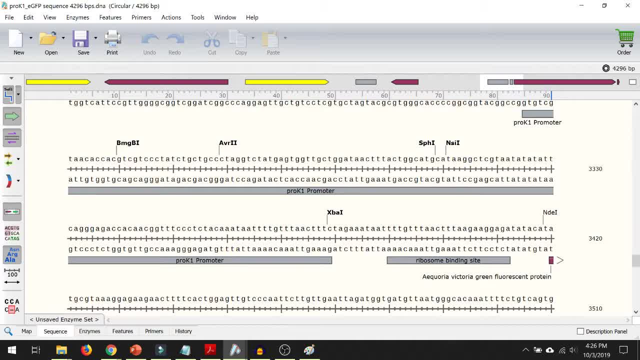 So you can sell it or use it or something. Now, after that is a ribosome binding site. Ribosome binding site tells the ribosome where to bind the mRNA. right, If you remember from last class, we talked about how the ribosome makes the proteins. 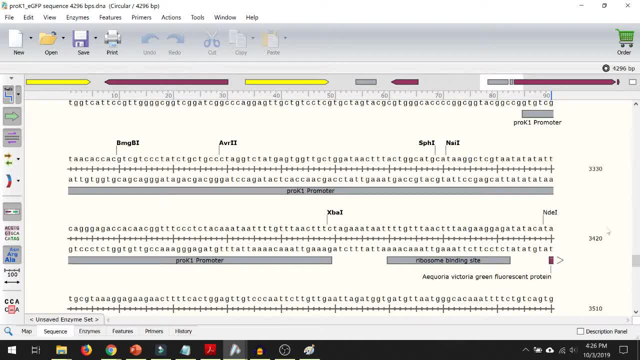 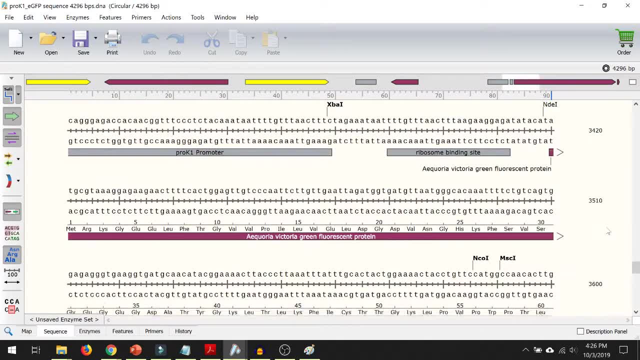 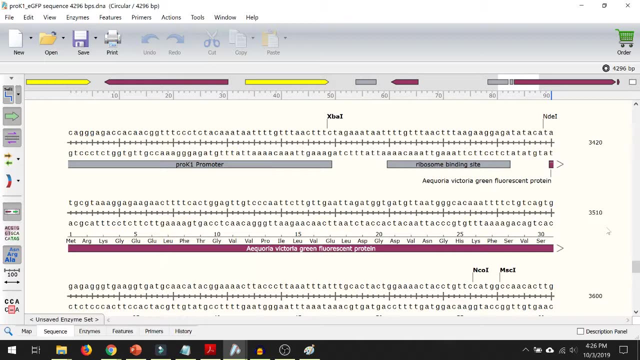 So the ribosome needs a binding site so it can make the protein That will become, or, yeah, we'll make the protein that is your gene of interest. In this case it's green fluorescent protein. Now I want to say every protein starts with a methionine and ATG. 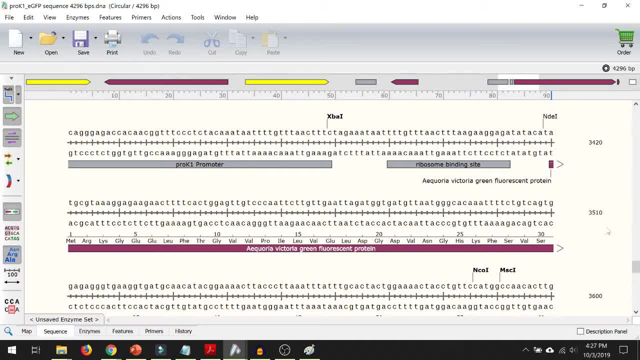 But, But it's not completely true. There are, you know, promiscuous stop codons that aren't methionine, And there have been a lot of data that shows that not all genes are started at methionine. But generally, when you are making a plasmid, when you're trying to express a protein or gene that you have, 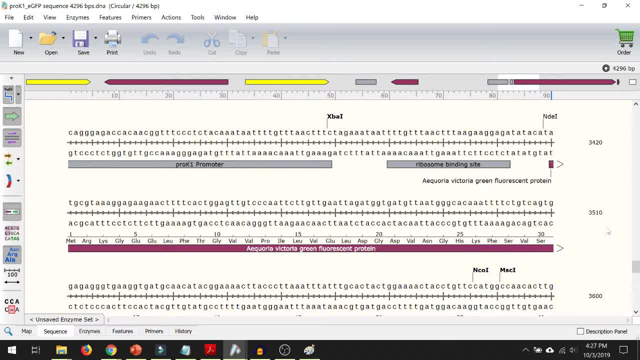 You're going to start Each protein With the methionine. you're going to use the start code on ATG, you're going to make the methionine And that will start The amino acid linkage together to form your protein. Now 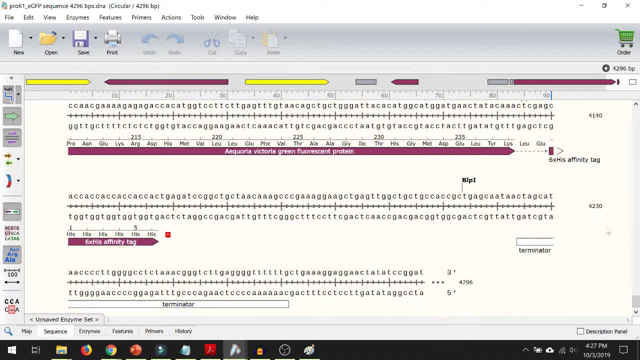 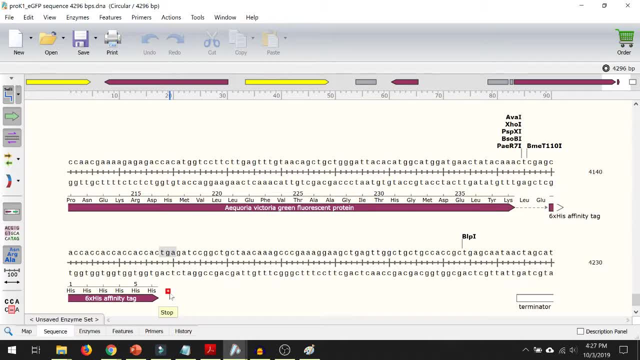 When you want to end your gene, You're going to have a stop code on here. you can see it by a little star. Generally That indicates the stop codon. So again, Generally You're going to use a stop codon. 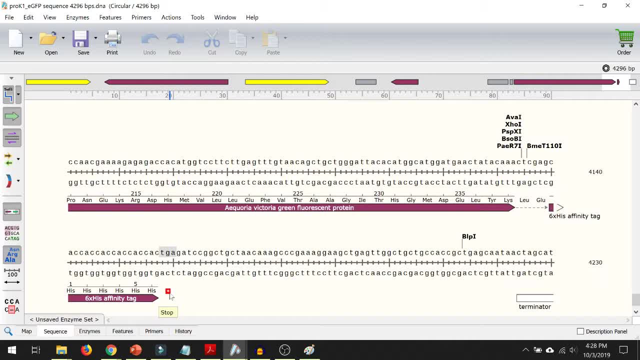 There is, I think it's three. Oh gosh, don't quote me on this. I haven't Looked at the codons lately, But there are a few different stop codons. TGA is One of them. Obviously, it's being used in this gene. 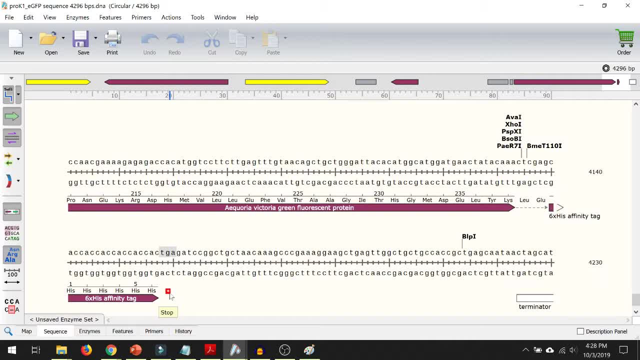 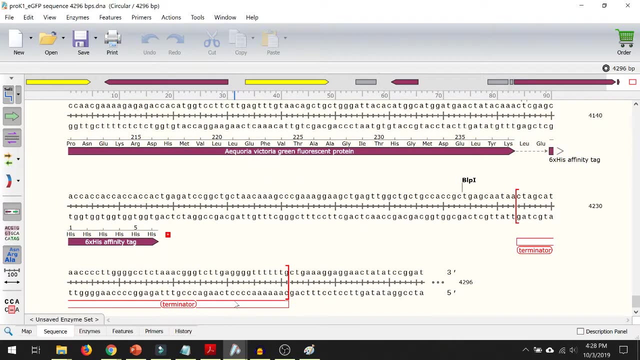 And it tells The ribosome where to stop adding amino acids, so that the protein is going to stop being made, right, But it doesn't tell something like the RNA polymerase where to stop. So generally, you're also going to have a terminator. so you're going to have a promoter and a terminator. 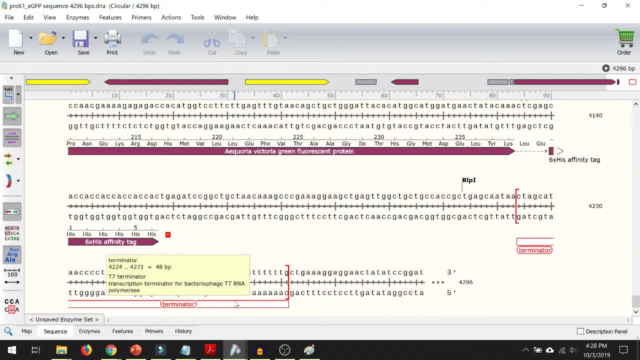 The terminator is going to tell Where Transcription, Where The mRNA, should stop Being made, Right? So like You have two different processes, You have the mRNA being made and you have the protein being made. Both processes Need to tell when to start and when to stop. 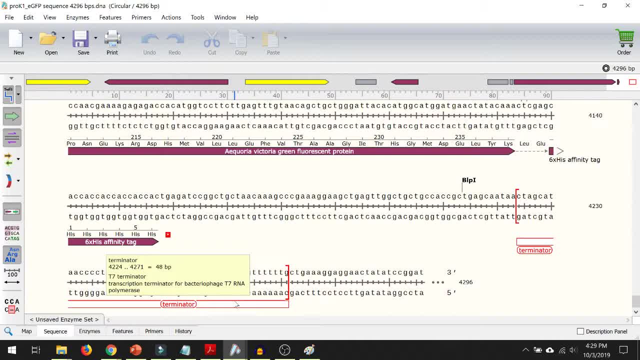 Right. So you could kind of think of this as like a Somewhat of a programming language. it's not a hundred percent exact like a normal computer programming language, because we're dealing with biological Things that have promiscuity based on thermodynamics. 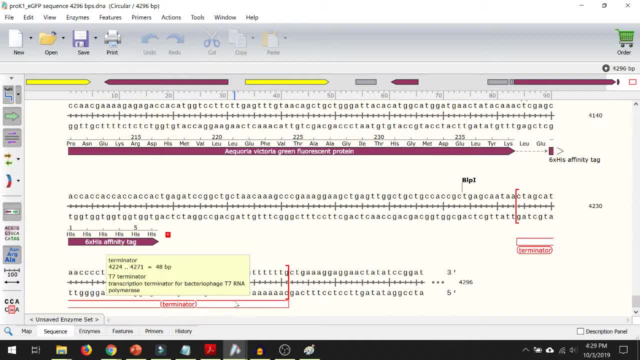 So it's not going to be a hundred percent exact, but it's going to have a high percentage of working this way. So both have the beginnings and the ends, and that's the important part to know Now. generally, when you insert a gene into plasmid, all that stuff is already in there. 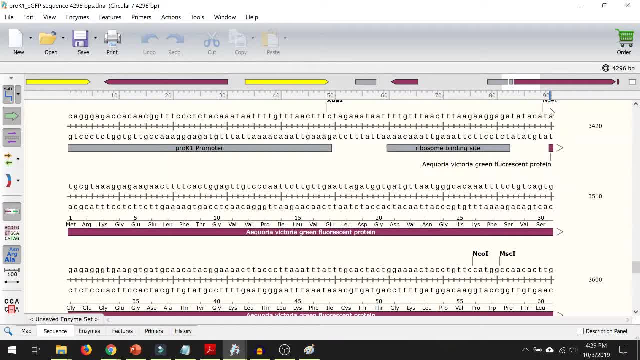 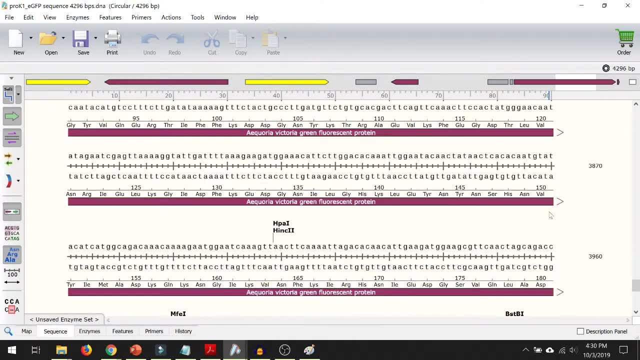 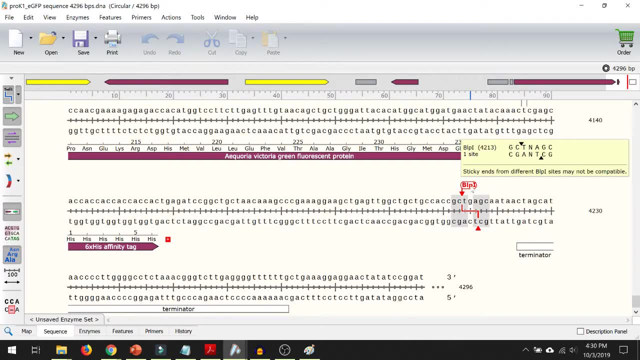 The only thing that you're adding to it Is the RNA Right. The only thing that you're adding is your gene. So you're going to insert your gene, Like something between This NDE1 site And This BLP1 site or something. 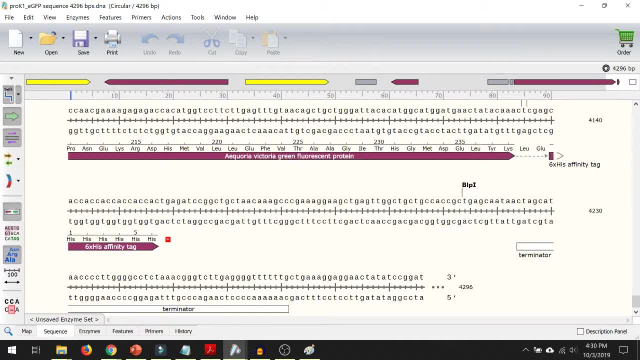 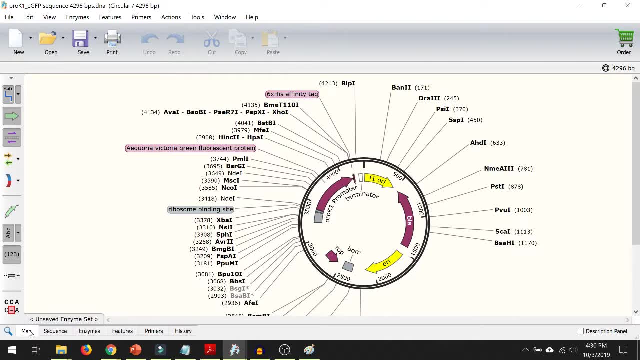 Now, what are these NDE1 and this BLP stuff? All right, Let's talk about that Now Instead. You know, Molecular biology is complicated and we're just starting to get to the place where we can Synthesize DNA on. 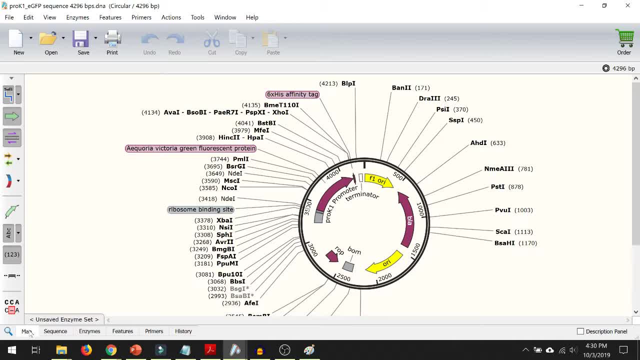 At a cheap enough price and a big enough scale, To where You know we can make a lot of the things we want. But that always has not been the case. It's not always been the case, Right? So There are these things that scientists discovered that are called restriction enzymes or restriction endonucleases. 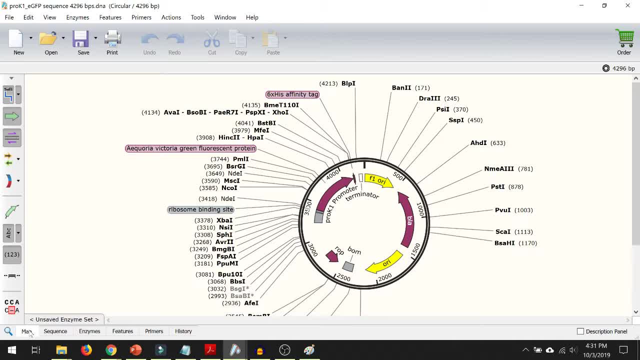 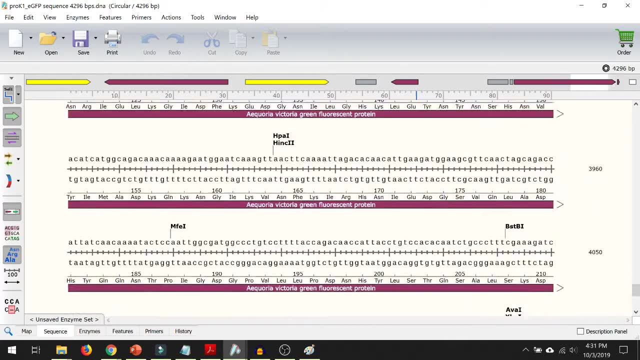 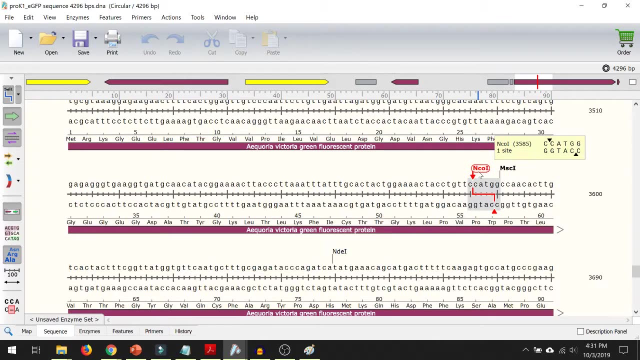 And what these enzymes do is they cut DNA at certain sequences, Right? So if we go back to the DNA sequence And We look at NCO1. You see it's highlighted, It highlights the DNA And it says NCO1 enzyme. 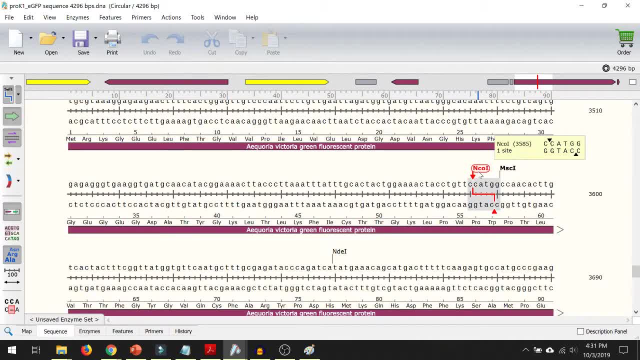 Will cut DNA at this specific sequence: CCA, TGG, Right. So It's going to cut DNA at this sequence And Every time, Almost every time, it's going to cut DNA at this sequence. So if you purify and add this NCO1 enzyme to your DNA, 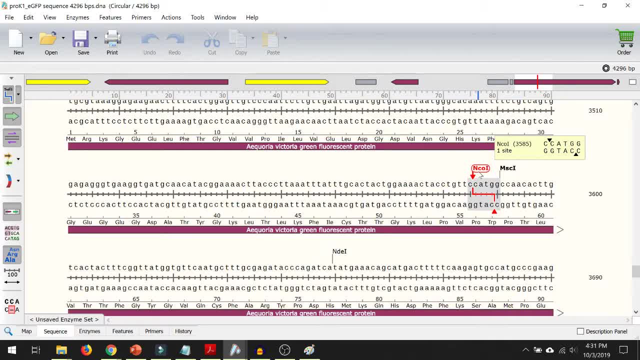 It's going to cut it at that sequence. Right Nowadays, we don't purify these enzymes ourselves. Companies purify them And they sell them to you. And then You know You, You just buy the enzyme from the company. But These enzymes allow you to cut DNA at specific places So that you can put DNA in Right. So If, Like I said, If I want to put in a new gene, I'm going to cut before the gene starts. 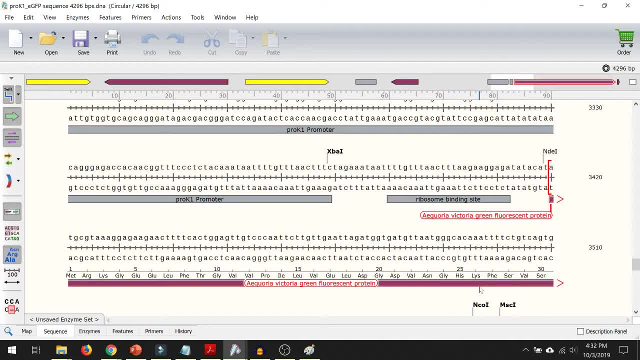 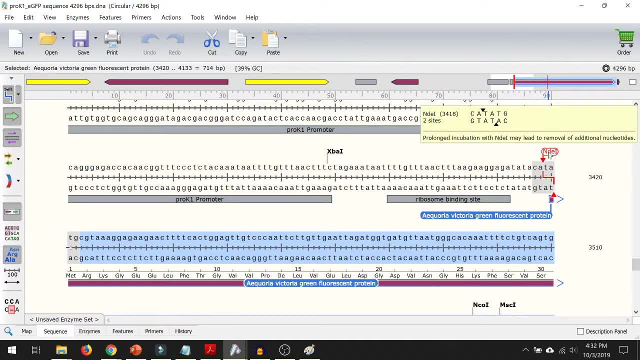 Right. So we have Our green fluorescent protein, Which is coded in the DNA, right here Now. The NDE1 site is CATATG. It's generally always used at the start of proteins because it has the ATG in it. 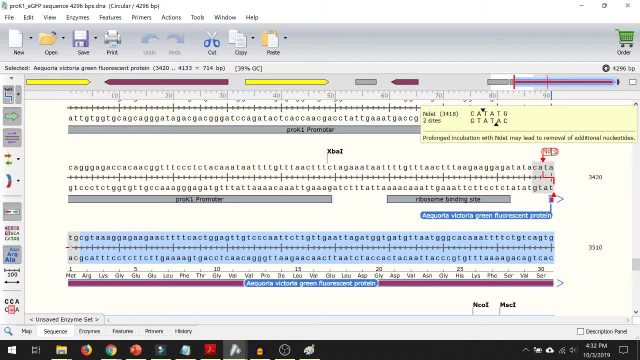 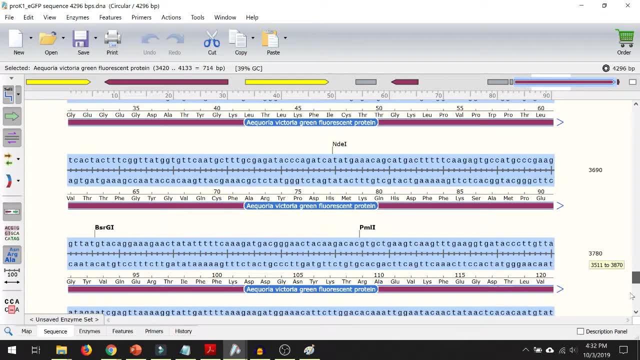 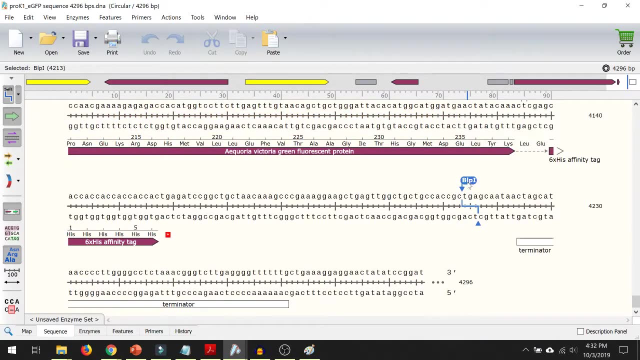 Right, And remember, ATG is the start, codon It codes for the methionine, CATATG. And then you're going to cut something that's after The protein Right, Like Perhaps this BLP1.. Or something. 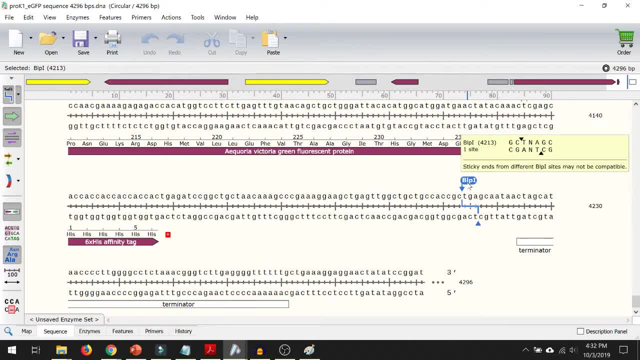 Right there Now, When the sequence has The restriction enzyme site Has an N in it. That just means Any amino acid, I mean Any Nucleotide. So whenever you see an N In DNA, It just means. 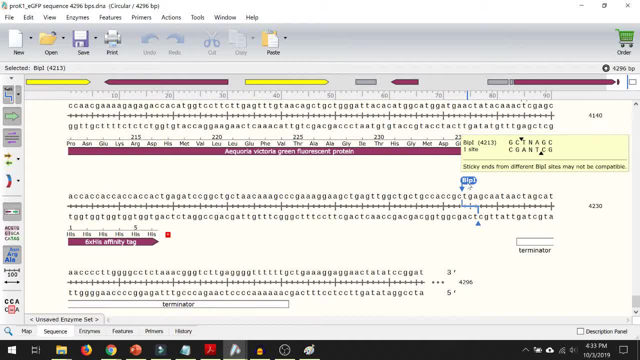 Any nucleotide N, Right, So This will cut at the sequence of G C, T, N, Right, So This will cut at the sequence of G C- T- N Nucleotide, And then. 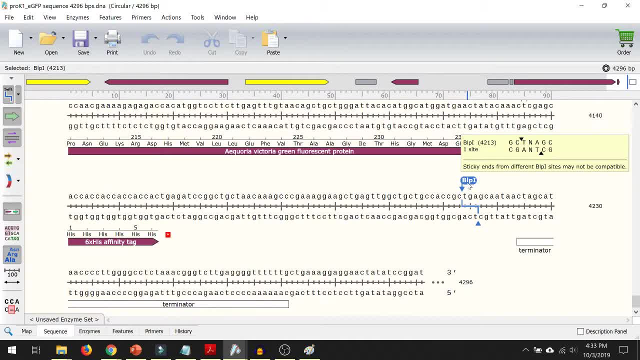 A, G, C. So that's the site Right, That's the site in DNA That this enzyme will Cut at And it will cut at Generally No other sites. So Once we cut the Our, The DNA, 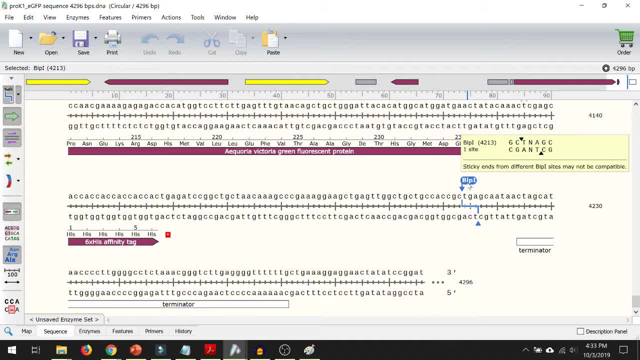 Out Of this plasmid. What we can do Is We can put In DNA That we have synthesized Our cells. That will match up And Get right in Like a puzzle piece, Right? So 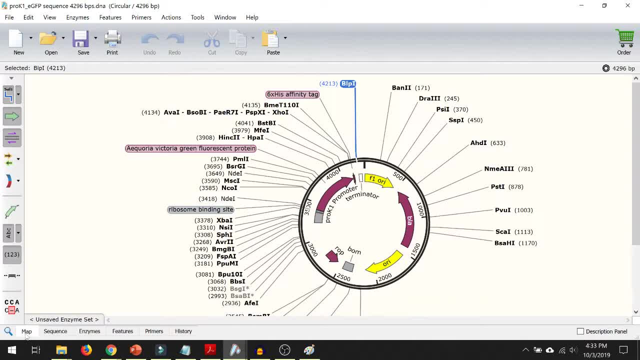 Now, If we look At The plasmid map, What you can see Is there are just A Ton Of Restriction Enzyme Sites Everywhere. These Restriction Enzyme Sites. 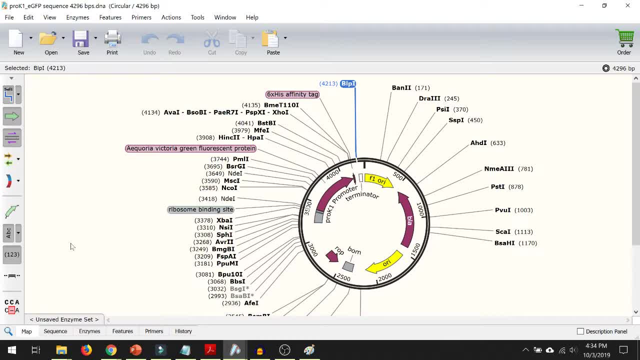 Give people The ability To kind of, You know, Pick and choose To do Insert Things, Cut things out. Now It's Super Primitive, Right, I get it. What you're doing Is You're. 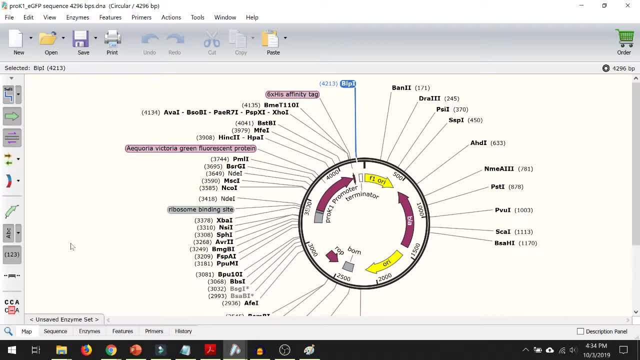 You're Literally Changing The DNA Just By Cutting Things Out And Putting It Back In. But You Have To Understand Also That A Digital System 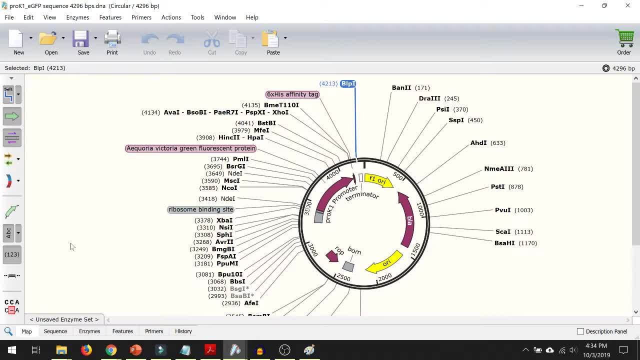 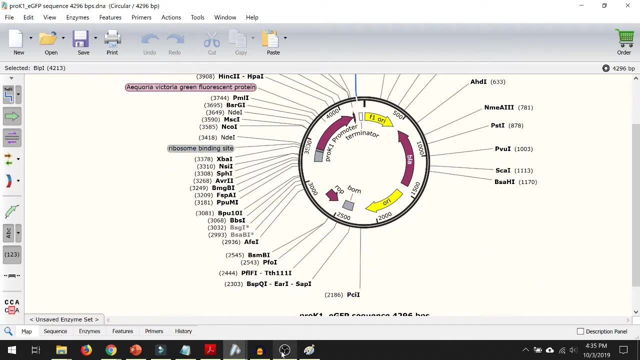 So People Love To Use Computer Analogies To Explain Biological Things. But It's You Know. Some Of Them Are Okay, But It's Not Quite. 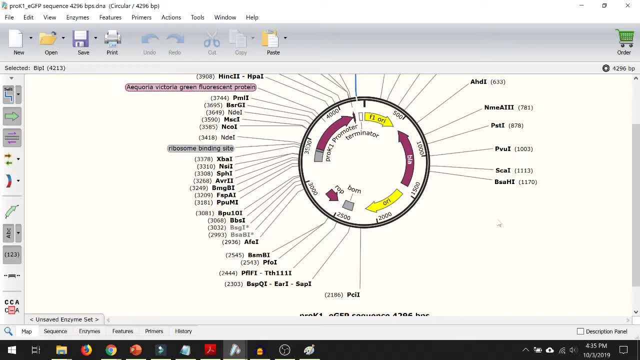 True, It's Not A Way To Change A Line In Code And It'll Change It No Like You Literally, If You Want To Change. 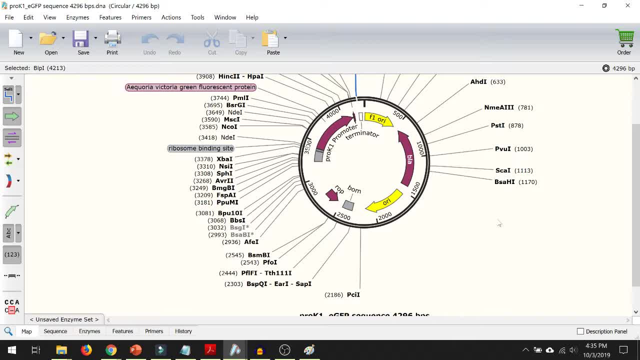 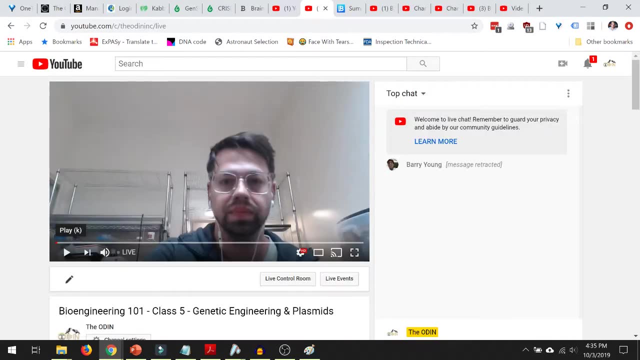 The Code. You Have To Remove Something To Use To Do Cool And Crazy Things. All Right, Any Questions? We Got Any Questions Here, Anybody? 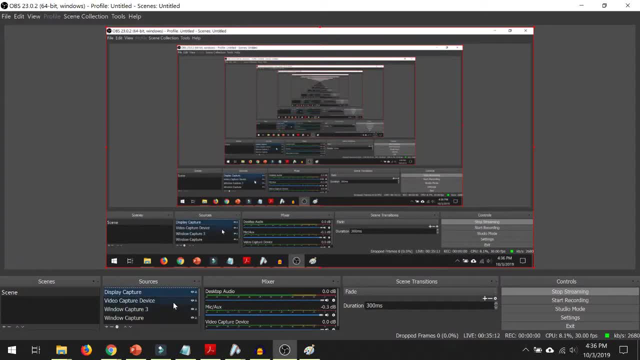 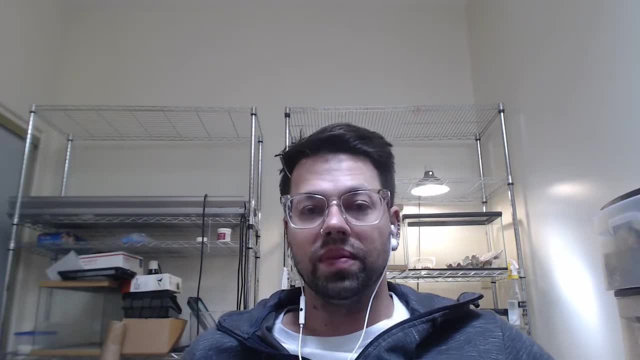 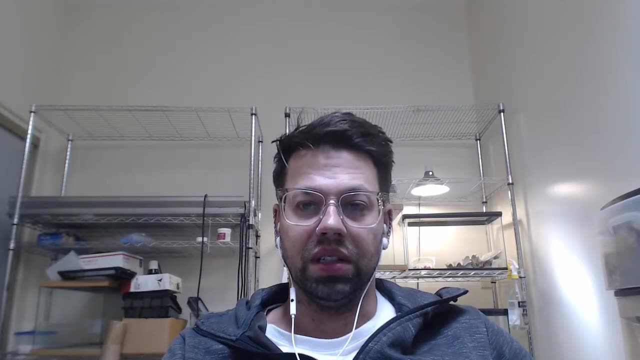 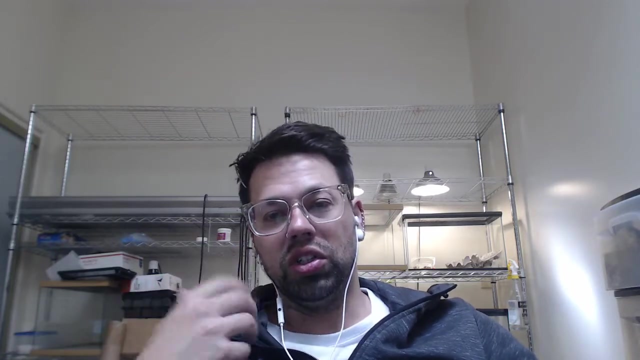 Barry, You Got Any Questions For For Me, What's Going On? We Got Questions, Questions, Questions. You Know This Is A Lot Of Stuff Throwing. 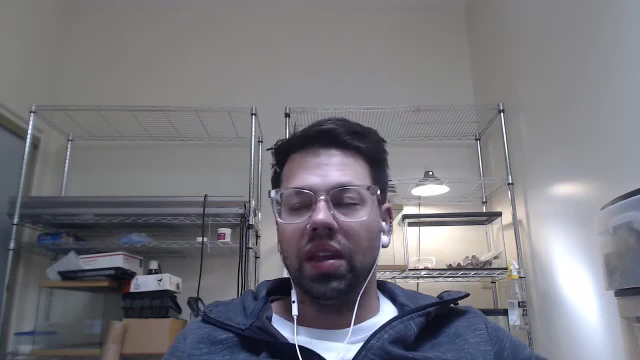 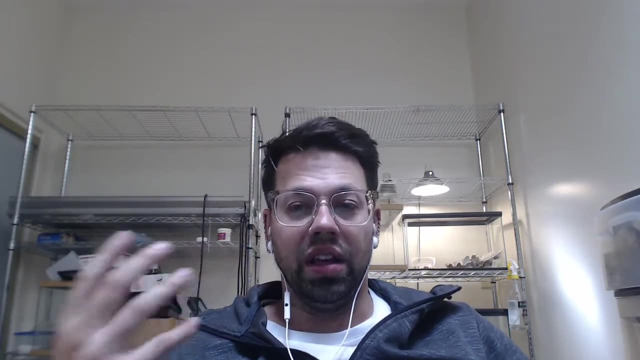 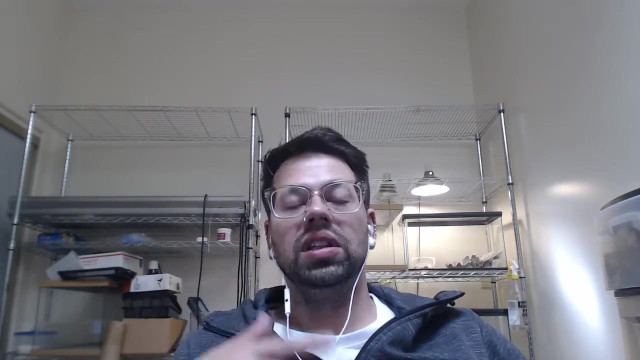 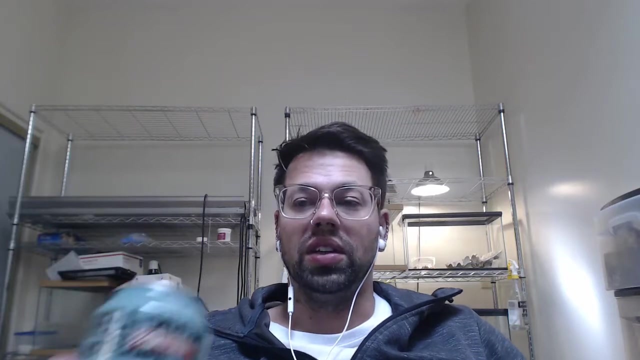 A Lot At You, But You Know, Try To Just Understand It As Much As You Can. You Just Need The Repetition, The Constant Repetition. 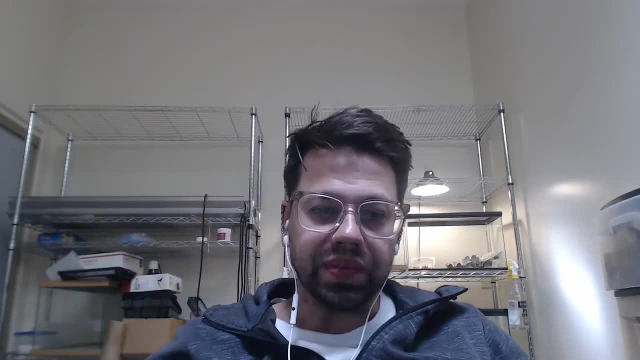 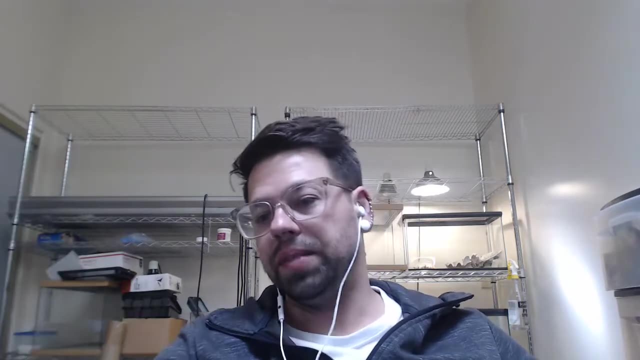 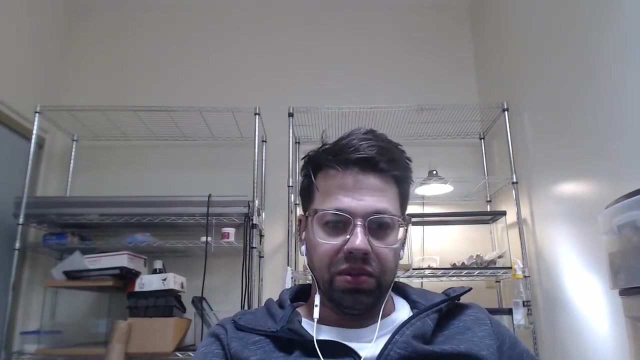 To Keep You Know, Forcing It Down Your Throat And Telling You How Things Should Be. Now The Experiment Is Going To, So Let's. 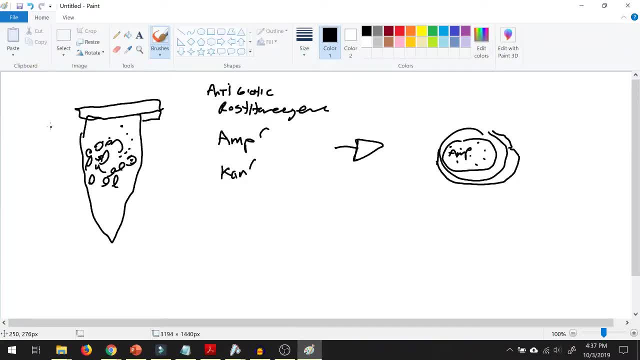 Go Over That Really Quick. So The Experiment You're Going To Do With Genetic Engineering Involves Adding, You Know, Obviously D N A Into. 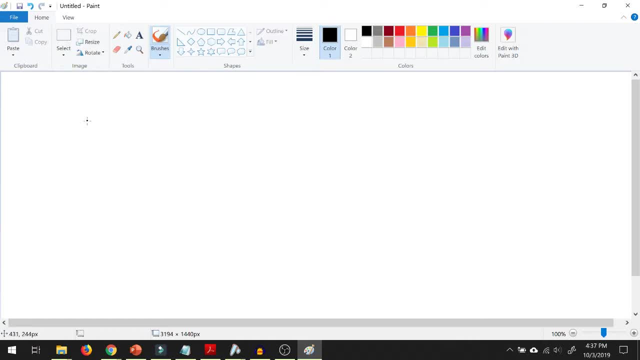 The Bacterial Cell. What You're Going To Do, The First Step One Is To Grow Up Fresh Bacteria, Fresh D, H, Five Alpha Bacteria. 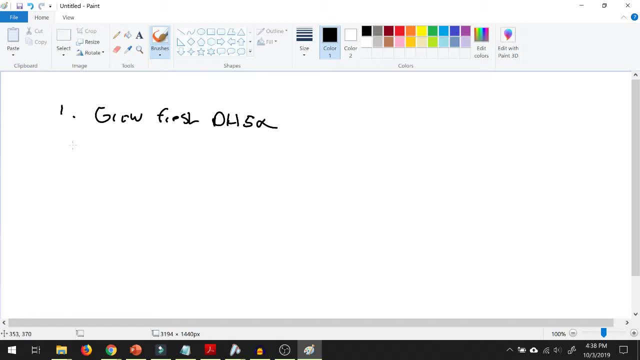 So Right, So Make Some LB Agar Plates. You Could Also Search It Online. To What You're Going To Do Is You're Going To 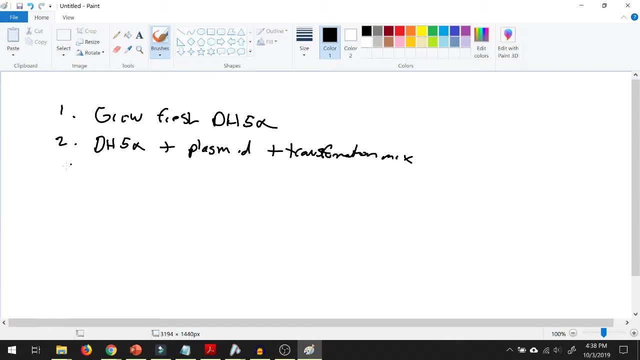 Mix Your D H Five Alpha Plus Plasmid Plus Trans Formation Mix Right, Remember The Peg Plus Calcium Chloride, Which Helps The Plasmid. 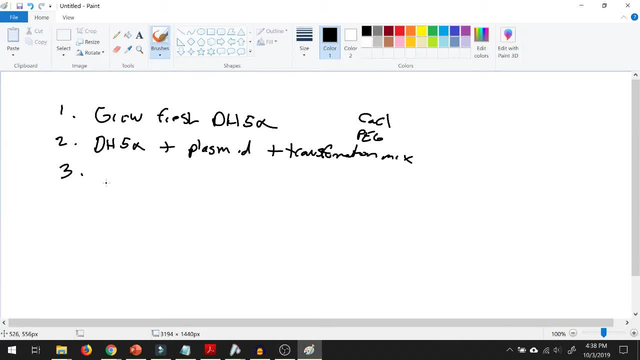 Get Into The D N A Now. What You're Going To Do After This Is You're Going To Try To Get Your D H Five. 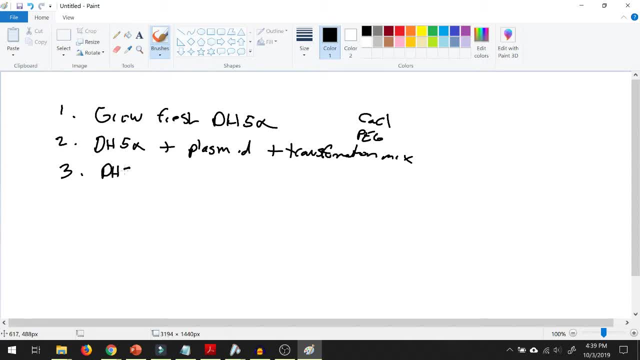 Alpha Plus Plasmid Plus T Mix Into, Say, Your Fridge For Like Ten To Twenty Minutes, Not Freezer Fridge Freezing Will Kill The. 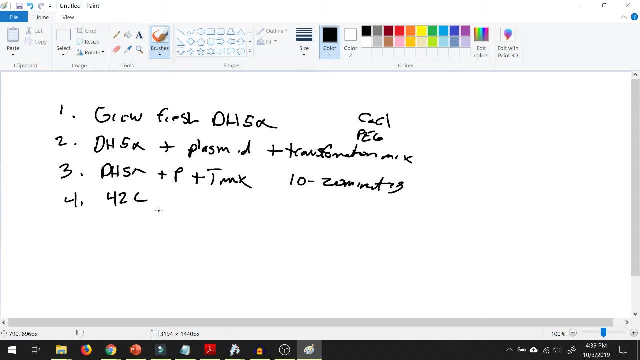 Bacteria. You Put It At A Temperature Close To Forty Two Celsius And This Creates A Temperature Gradient. Heat Shocks The Bacteria And Helps 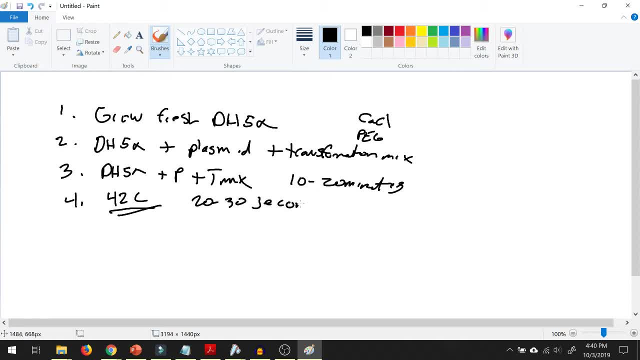 The D N A Get Inside Your Bacteria. So Be Patient, Just Sit There, Count Out To Twenty And Then Take It Out. It Doesn't. 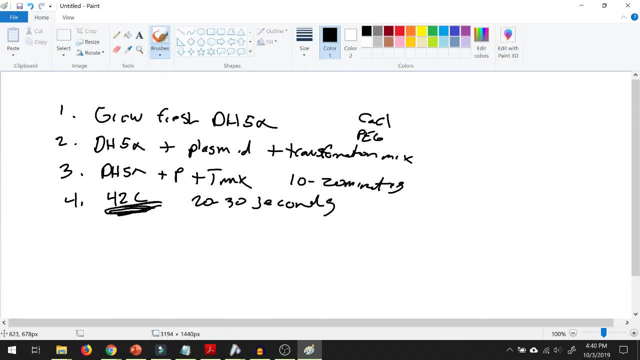 Have To Be Exactly Forty Two Celsius. Either You Know, Is A Little Bit Of Heat Shock To Help This Happen Right Afterward. What You're Going To Do? Is You're Going To Help The Bacteria Recover, Right, So We Let The Bacteria Grow, So You Want To Put Them? At You Know 37. C, If Possible Comfortable Temperature For Bacteria Where They Like To Replicate Fast, Or If Biotic Selection Right. So 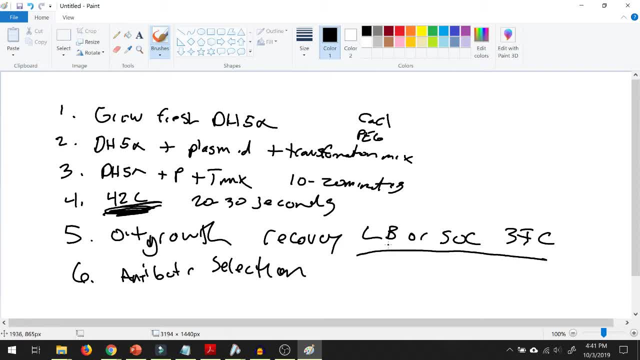 After Your Bacteria Have Taken Up The Plasmid, They've Started To Replicate And Recover. Then You're Going To Put Them On Antibiotic. 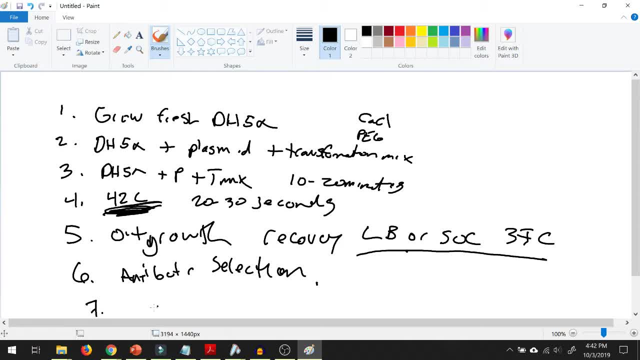 Selection Plate By. You Should Have The Bacteria With Plasmid. It's Not Always The Case. Sometimes You Get Contamination Or Something Else. But That's Generally What Should Happen. Bacteria With Plasmid At Human Cells You Don't Do Any Sort Of Heat Shock, But Basically Everything Else. 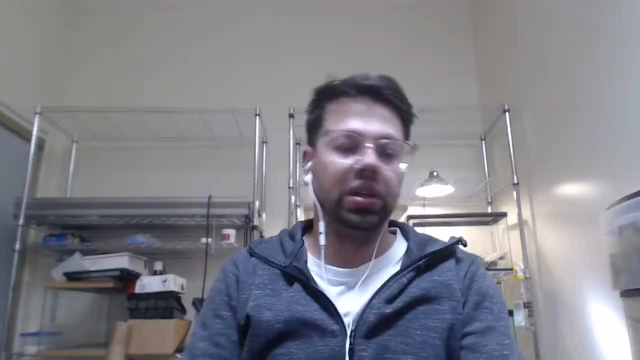 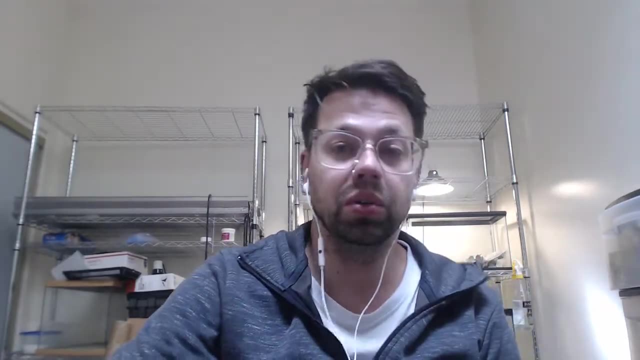 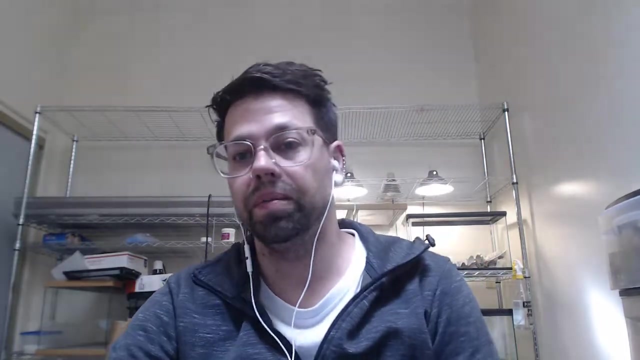 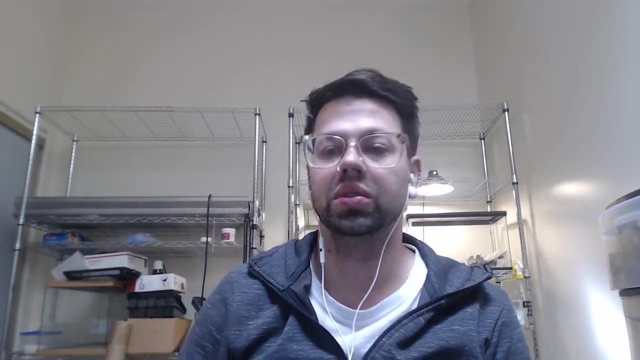 Is Really Similar. All Right, So Get On That Experiment This Week. Do Your First Best To Answer Those Questions. Barry Has A Question. He Said. 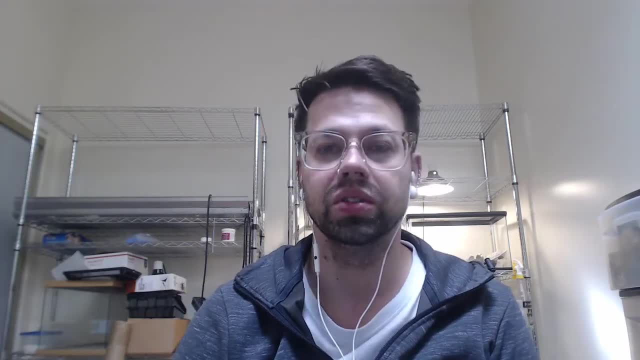 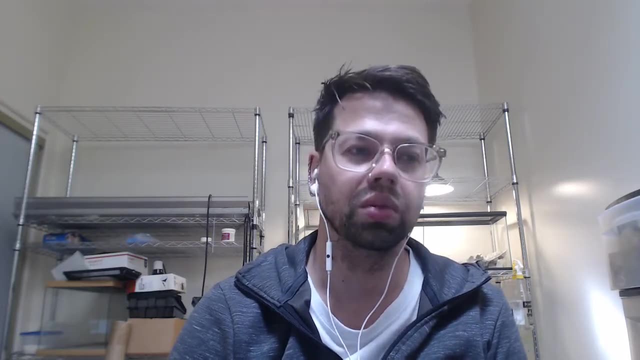 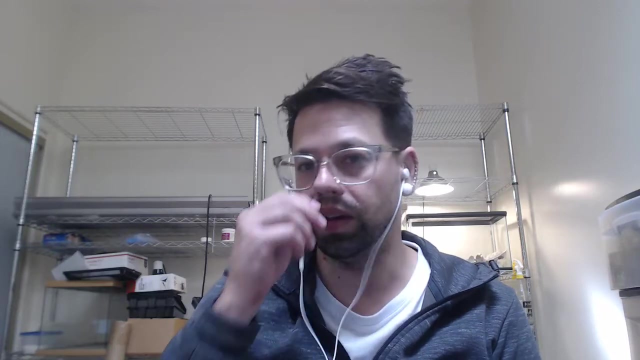 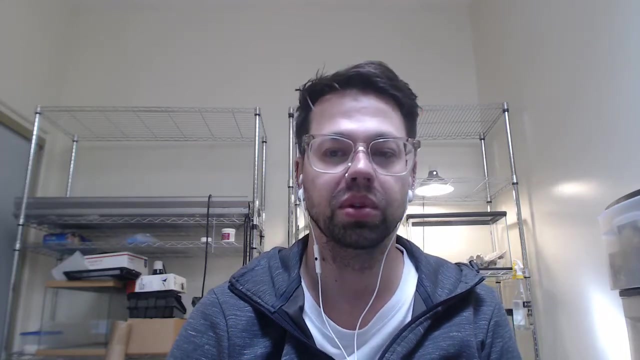 How Do You Choose What Promoters, Origins, Etc To Use? I Know There Are Quite A Few Generally, You Know Once You Get To That. 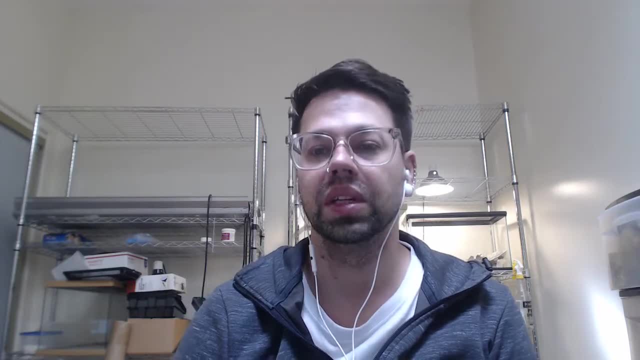 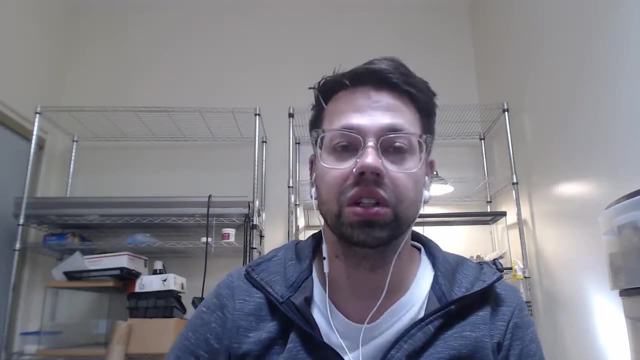 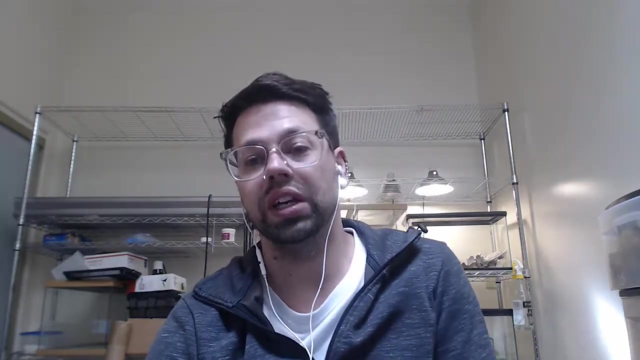 Place We're Starting To Use: Promote, Choose Promoters And Origins. You'll You'll Know, You'll Have An Idea Of What You're Trying The. 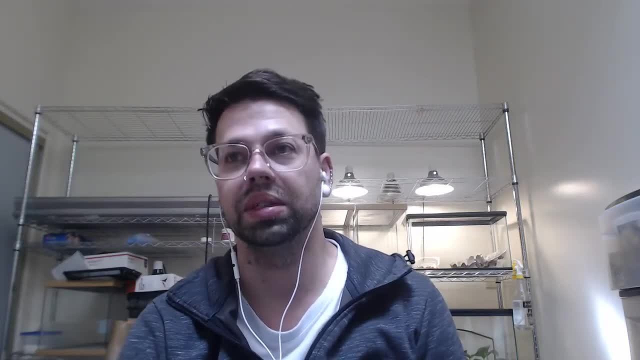 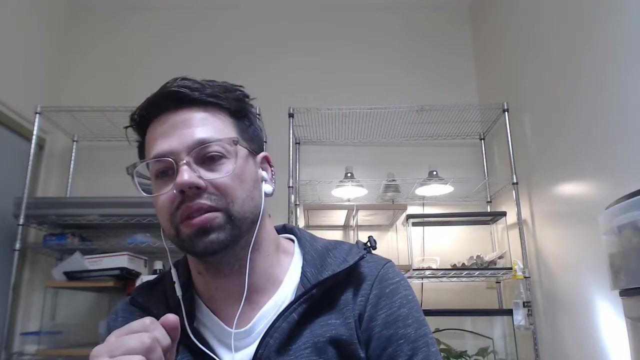 Bacteria- The Majority Of Bacteria- Are Not Going To Receive The Plasmid, So Your Ability To Find Bacteria Or Whatever Organism That Have